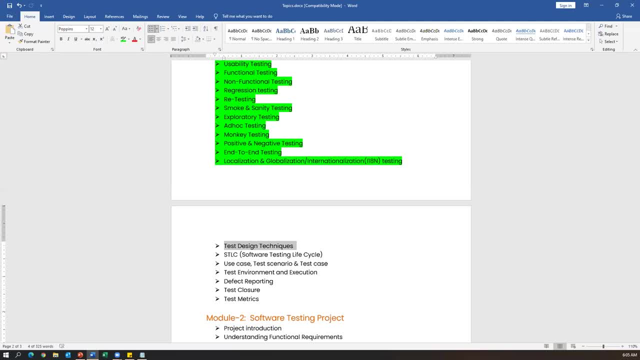 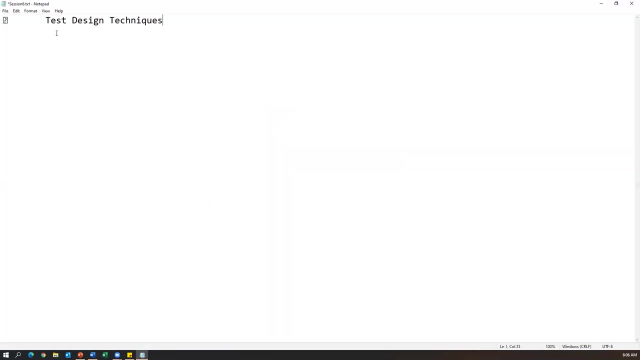 contains the spaces, username contains a special character, username contains the numbers or username contains a combination of numbers and alphabets. So different type of data we have to prepare And then we'll conduct the testing. So what test design technique will be used? So the test design techniques will be used to prepare the test data. Okay, so let me write small notes here. We can say test design techniques or test data or test case design techniques, whatever it is. 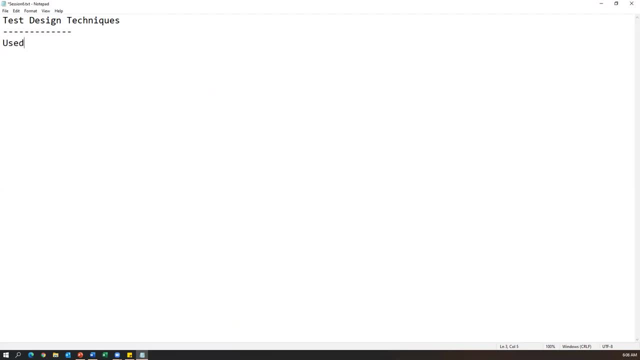 So the test design techniques will be used to prepare data for testing, for testing, And that is the one thing. And the second usage is sometimes to test some functionality. we have to prepare so much of data. So instead of preparing the so much of data, we can minimize the data and we can improve the coverage. there are two things are important. The first thing: 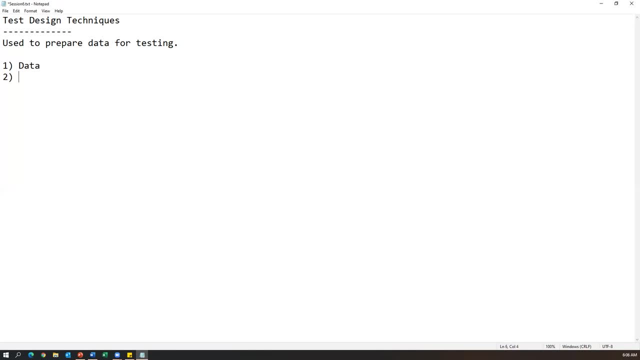 is data and the second part is a coverage. so what is data means? the data means which is used for testing and what is coverage means whatever data we prepared, with that data we should able to cover all the scenarios of testing. so, for example, again take the login functionality. so valid username and 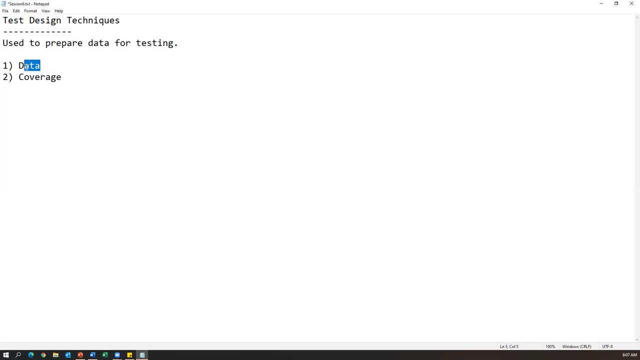 valid password or invalid username. invalid password or valid username, invalid password. so different combinations of data we have to prepare. and while you're preparing the combinations of data, because we have to cover all the scenarios, all the testing scenarios, so that is called as a coverage. okay, so the main usage of test design techniques is to prepare the test data which will. 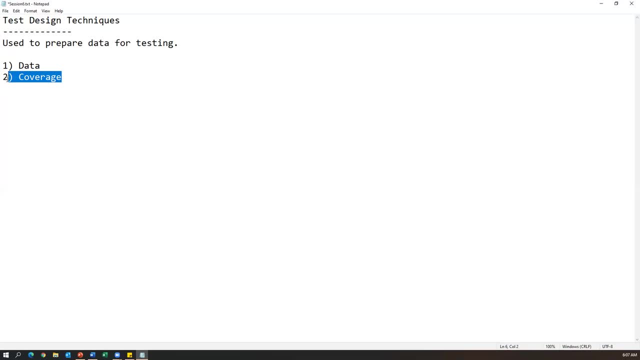 cover each and every area of the feature, which will cover the each and every area of the feature, every of the functionality we can you cover. so that is the main intention of using test design techniques. so by using test design techniques, we prepare some test data which can cover each and everything of the functionality. 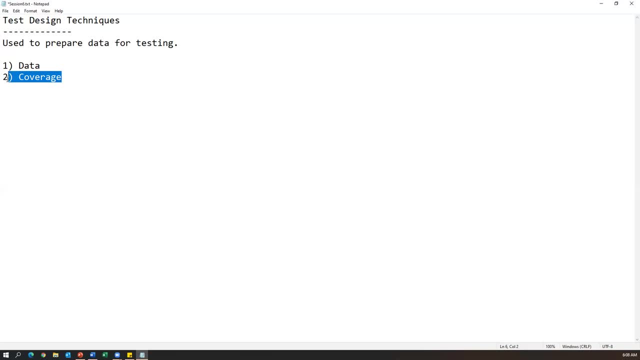 so that is the main usage of tested design techniques, and by using tested design techniques we can also reduce the data. with minimal data we can cover everything. okay, for example, i have a small- let us say i have a simple or a small- text box. okay, so in this text box i just want to enter age of the person. okay, so my 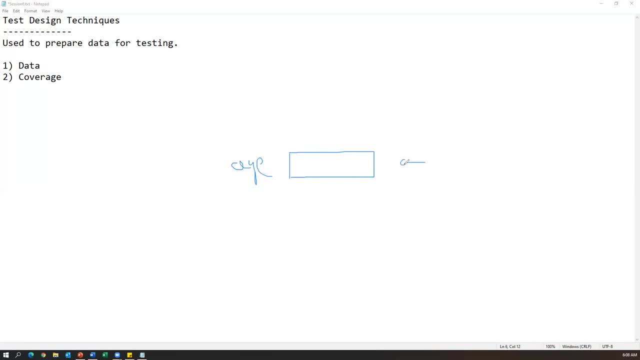 requirement is the age should be in the text box allows. age should be, let's say, 18 to 30 years. 18 to 30 years is my requirement. so in this particular requirement, how much data we have to prepare normally, how many inputs we need to test this? we have to test first of all how many inputs we need. 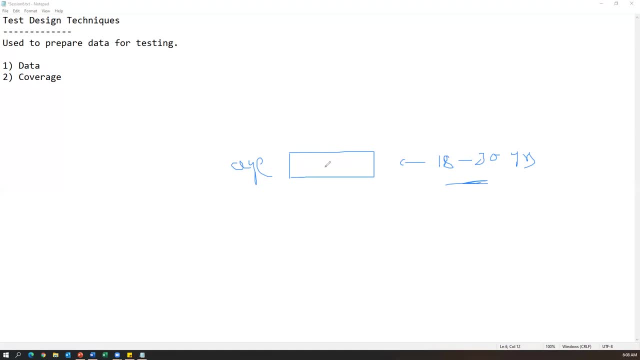 to test this. we have to test first 18, then 19, 20, let's say from 18 to 30, all the numbers we have to test, and these are all valid inputs. and below 18, whatever numbers we have from 1 to 18 also, we 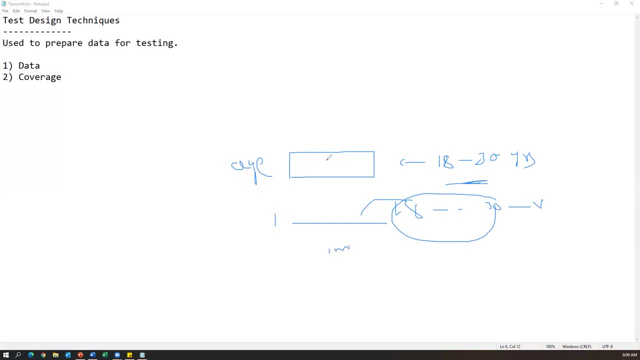 have to test. they are invalid data we should not allow. and after 18, after 30, whatever numbers we have, we have to test with all the numbers. these are all also input invalid data. so if i just look at the small requirement, there are huge data we have to test instead of testing all these kinds. 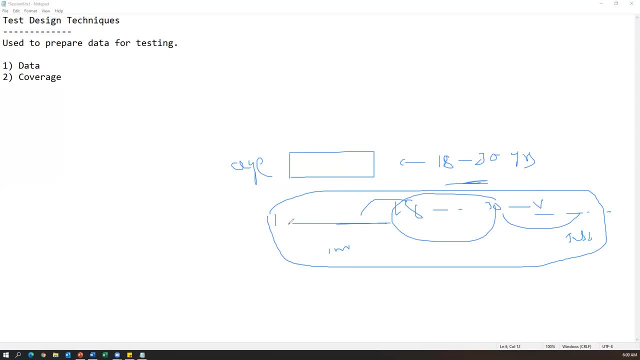 of data. we can just minimize the test data. we no need to go for all the numbers. by using testing techniques we can reduce the data, but at the same time we have to make sure everything is covered or not, each and every corner scenario also tested or not, with minimal data. 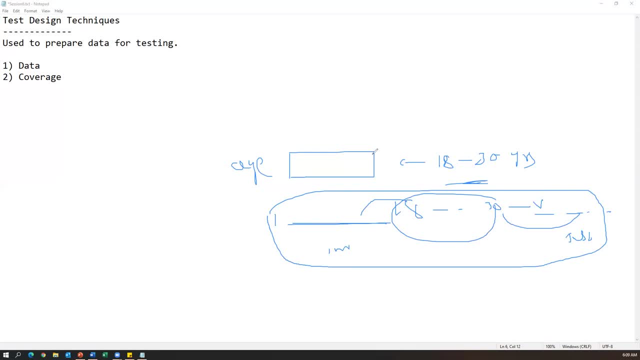 and the tested design techniques will be used there. so test design techniques will be used to reduce the data and more coverage. okay, tested design techniques will be used to reduce the data and also, which will increase the coverage. now let me write the notes. it will basically reduce the. 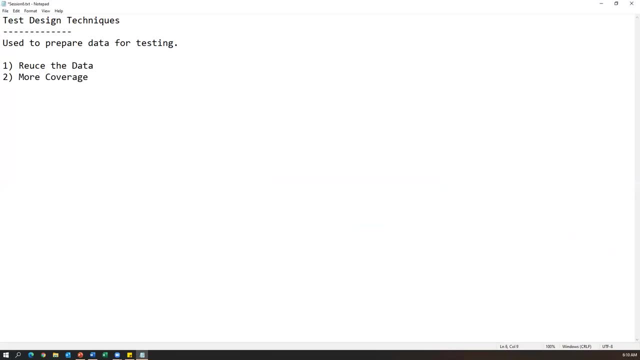 data and more coverage. so these are the two advantages of tested design techniques. but what are the test design techniques we have? so we have five types of techniques to design the test design techniques: equivalence, class partitioning, boundary value analysis, decision table based testing, or we can say decision base addition table, state transition, error guess. so these are the five techniques we 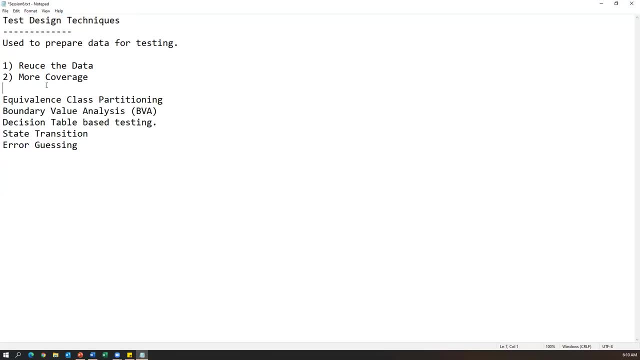 have. so these are called test design techniques, very important in interview point of view also, and especially when you go for ihdqb certification examination, you will get a lot of questions on this topic, so listen carefully. so these are the five types of techniques we have. these are called: 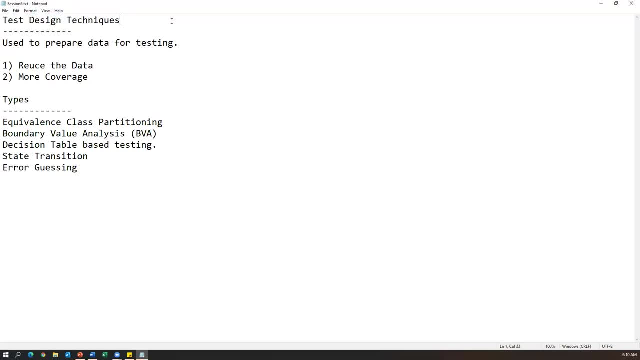 test design techniques, or we can say test data design techniques. okay, test data design techniques. or we can say test case design techniques. anything is fine. and what is the use of test design techniques? we can reduce the data and also we can increase the coverage. now let us discuss one by one. so there, 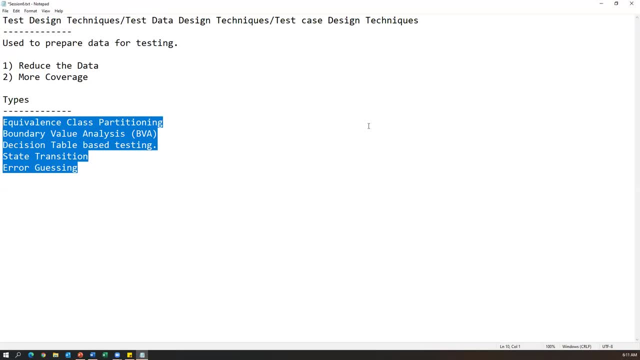 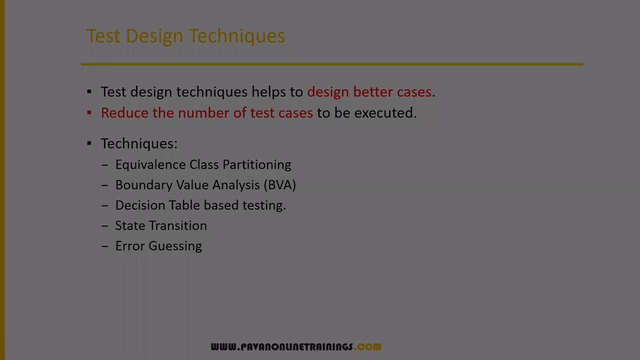 are five types. we have five tested design techniques: equivalence class partitioning- this is also shortcut called as ecp- equivalence class partitioning, boundary value analysis, bva decision table testing and state transition error guessing. so these are the five techniques we have. so now let us discuss one by one. so let me share small presentation just a second. 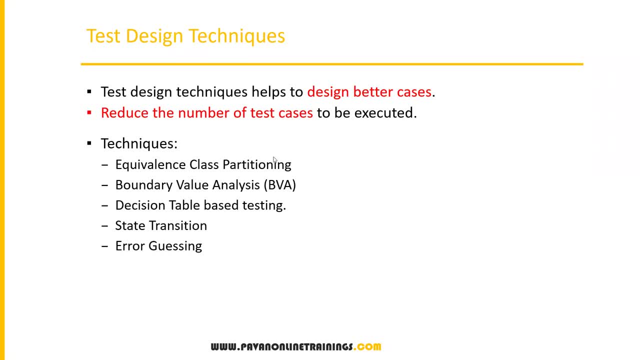 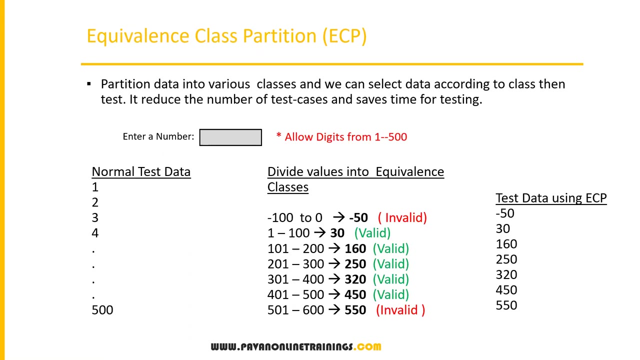 okay, so now, yeah, these are the four techniques. we have equivalence class partitioning, boundary value analysis, decision table testing and state transition error guessing. so there are five error guessing. so first let us start with equivalence class partitioning, so how we can use this technique. so here we have to mainly partition the data into various classes. 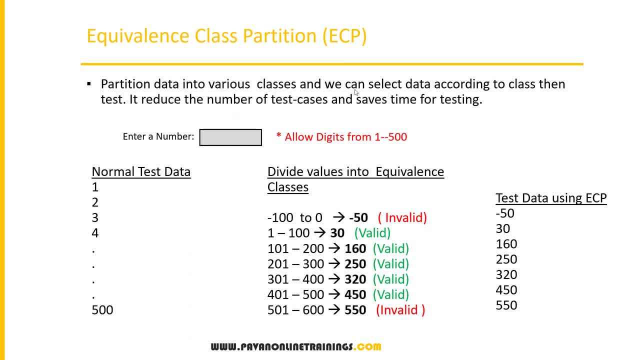 and we can select the data according to class, then test it, so it reduces the number of test cases and saves a lot of time. so i'll give you an example how it will reduce the data and it will cover everything. so let us say, this is my small text box. i have and i have to enter some 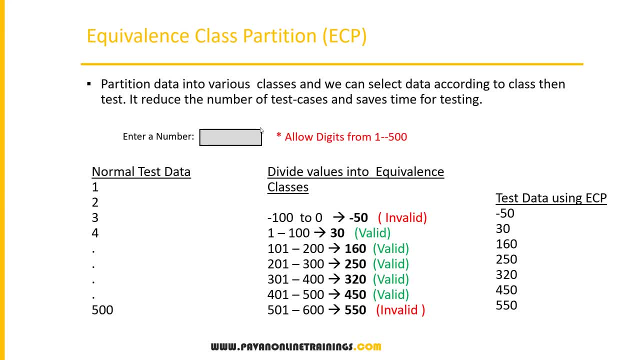 value in it and which will allow only digits, only numbers between 1 to 500. so i can enter only 1 to 100 values here, right? so if i, if i don't use any test data technique, right, how, we will test this with all combinations means we just try to enter from 1 to 500 numbers, so we'll test first one. 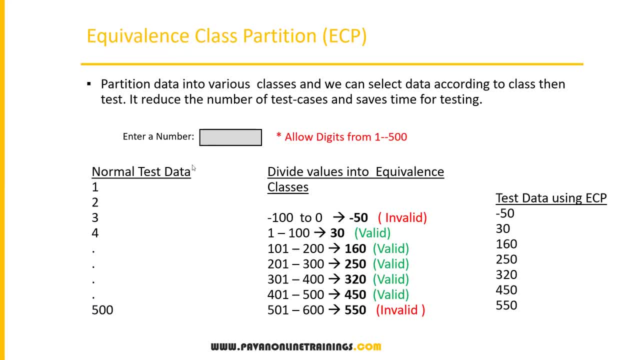 we'll check whether it is allowing or not. then next two, three, four, five till 500. so one, two, five hundred numbers we have to enter and test whether it is allowing or not. so that is a normal test data, okay, and instead of testing all the numbers, we can just use equivalence class partitioning. 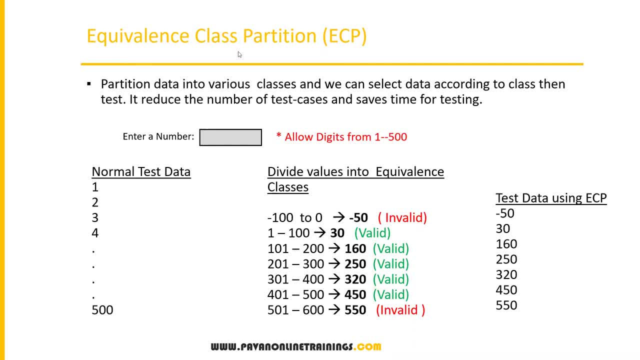 technique or ecp technique, and we can reduce the data and at the same time we can cover everything. so we don't need to miss anything here. with small set of data we can cover each and everything, all the scenarios. now let us see how we can use equivalence class partitioning technique to 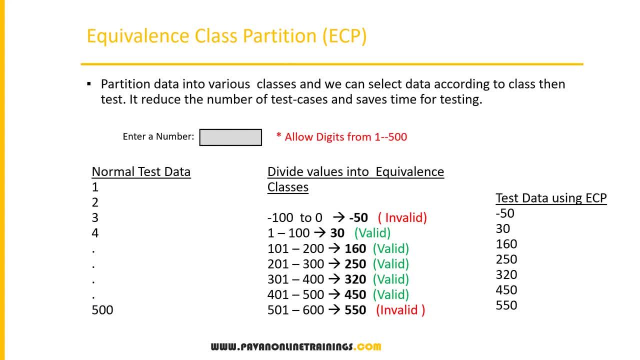 test this or to prepare the data. so if i just look at here in equivalence, class partitioning, what you will do is, as a first step, we will divide the entire data into multiple classes. okay, or we can say partitioning, dividing or partitioning, so partitioning data into various classes. this is the first step we will do. 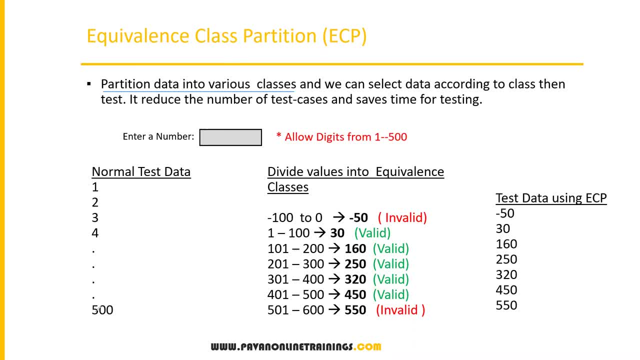 so how we can partition the data. let us say, i have one, two, five hundreds are allowed. so before one also we have to test some numbers, because that is invalid data, it should not allow. and after 500 also, what are the numbers we have? that is also should be tested, it should not allow. 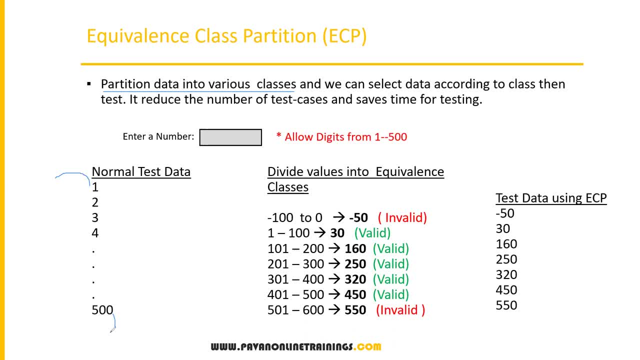 us, that is a negative data, so we shall also include them. so we have to divide entire numbers into the class. let us say: or we can place it down into the class or we can partition them. so in ecp we can say: divide values into equivalence classes. let's say: 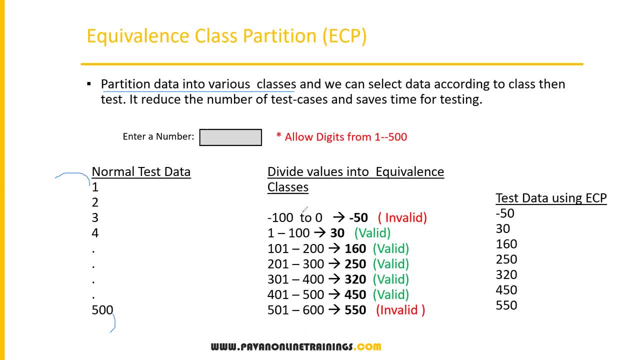 100 to 0 means these numbers are fall under below 0. okay, and let us take one number from this. from 100 to 0, take any one number. let's say i have taken 50.. and when i add this value here, minus 50 is not allowed- what does that mean? whatever number we have given in this range, 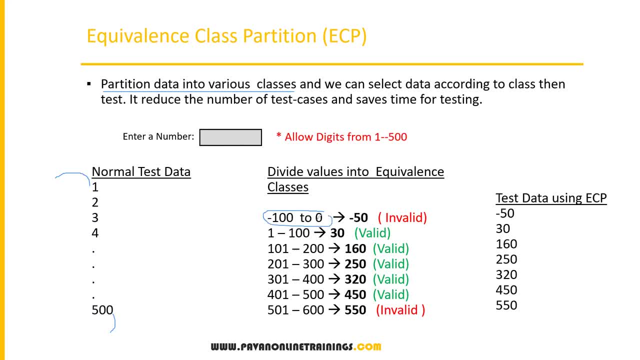 that should not allow. that will not allow, first of all. but we no need to verify with all the numbers. just take one value between this range and check it whether it's working or not. so if it is not allowed, means what? whatever number fall under this bit, in this range, which will not allow. 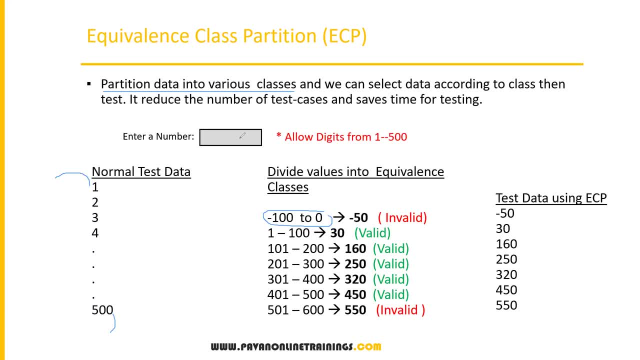 with which single value we can test that similarly: 1 200, 1 0, 1, 2, 200, 2 0, 1, 2, 300. so we will divide entire data into multiple classes. these are called equivalence classes. so once you divided, 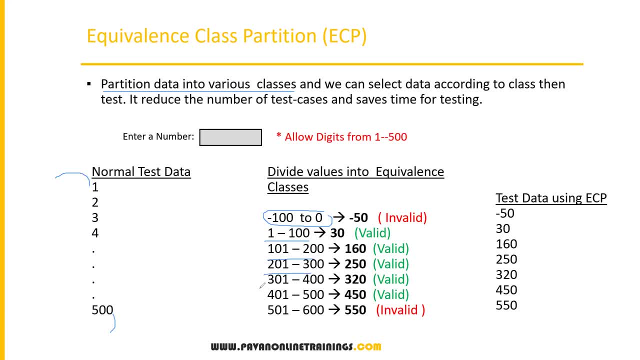 now, in each and every class, every group, we will take one value, let's say from 1 to 100. let us take 30, anything, any number you can take between 1 to 100. so if 30 is allowed means what we will test 30 here. 30 is allowed means what, which will allow all the number from. 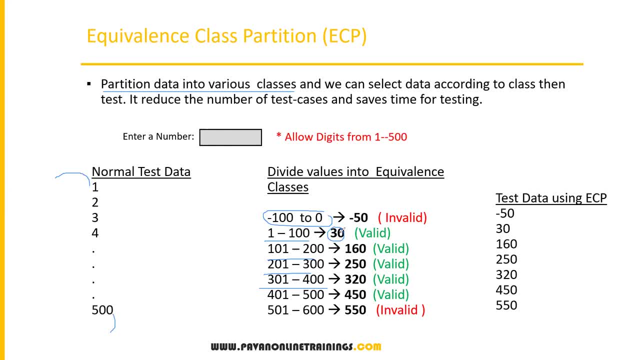 1 to 100. so just we are testing with one value. we no need to test with all the numbers 1 to 100, just take one value from that class and then test similarly: 1, 0, 1, 2, 200, 2, 0, 1, 2, 300, 3, 0, 1, 2, 4. 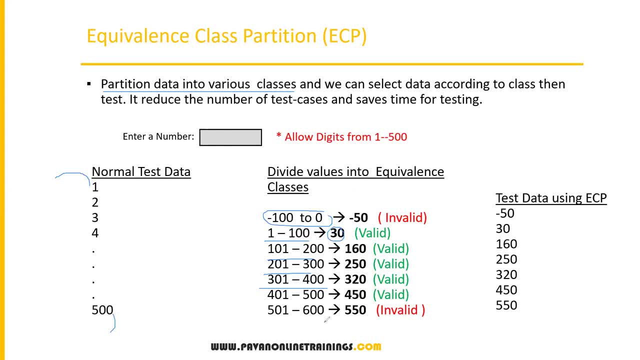 4 0, 1, 2 500, 5 0, 1, 2 600. so after 500 we will take one more class, because this fall under invalid data, so we should take one more class. so now, in each and every class we will pick one number, any. 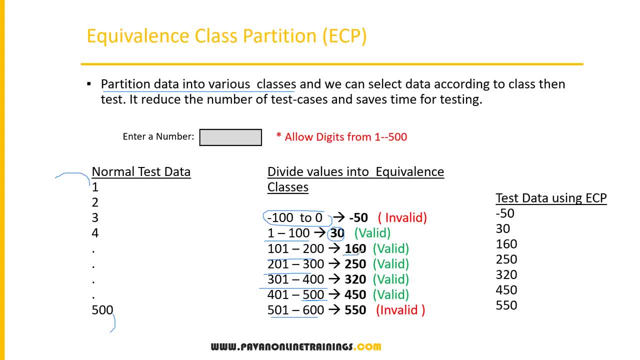 number you can take between that number. so here i have taken 160, which will fall under between 1, 0, 1, 2, 200. 250 again comes between 2, 0, 1, 2, 300 and so on. so from 501 to 600 i have taken 550, actually this. 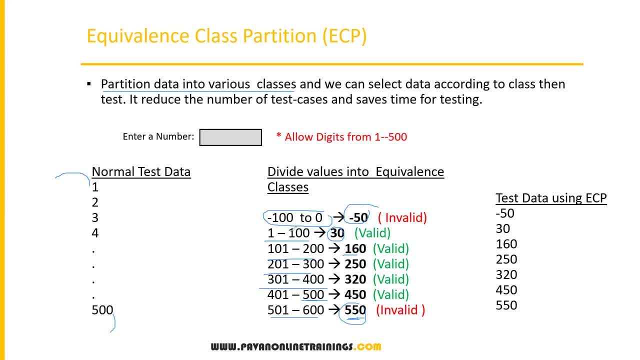 is invalid data. this is invalid data because we need to also test the invalid area. so this is how we need to divide the entire data into different classes and we'll choose one value from each class and these values only we will test. so if i just look at here, this is the final data which we are going. 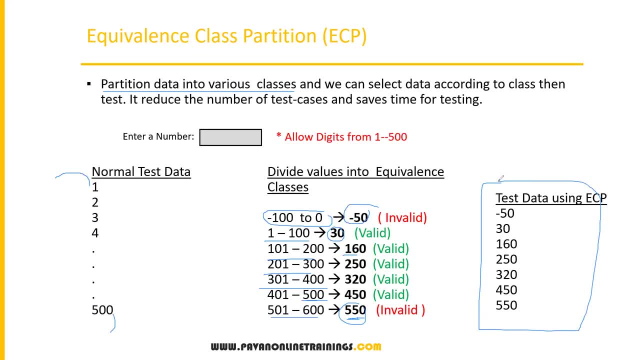 to use for testing by using ecp technique. so what ecp technique has done here ecp technique is covered everything at the same time. it reduces the test data. so we no need to verify all the numbers from 1 to 500. not at all required. 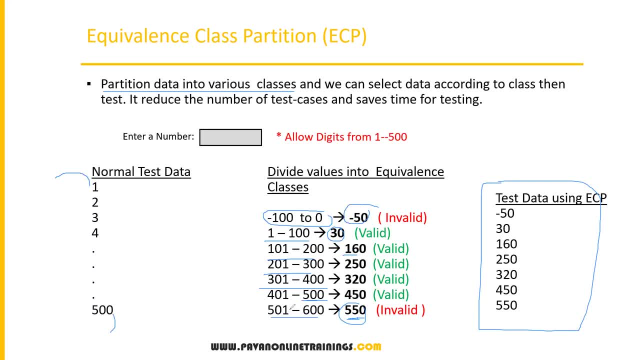 so here in each class we have taken 100. my lower level the number is a bit lower, but you know, known the numbers from each class are actual numbers in the process and to test the KNOW level. but in our case we will give 100 number, so we will just let it be 100 for the 2008 test case. so 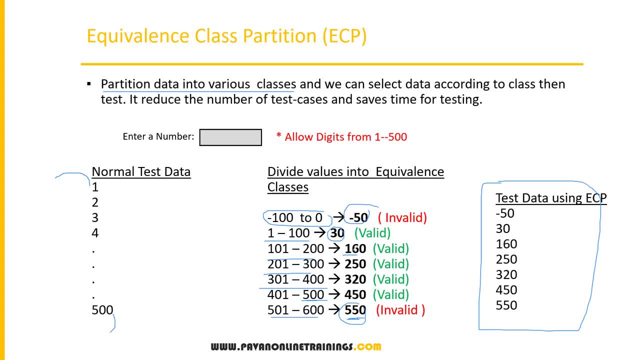 we have taken 100 only from 100 and i give a � to eq to 100 and so on to come with 100 now let's put some moreDerived data so for this mass lack numbers as you will see we have taken 600 but it is容ents by weightscationmultiplicate 음 and each and every class will pick some value 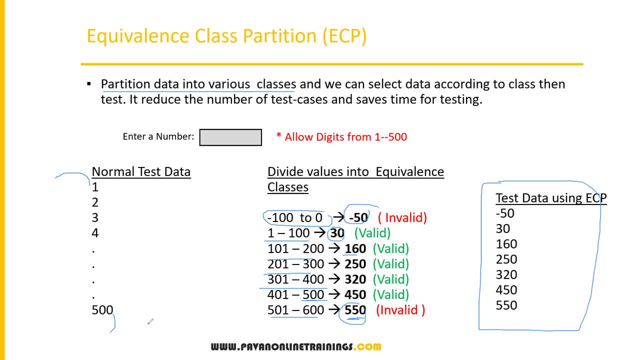 technique. so if i don't use this technique, we have to use all the numbers, every number we have to test again, which will take a lot of time, also unnecessarily. and here, by using ecp technique, we can minimize the test data. at the same time we can improve the coverage, test coverage. so that is. 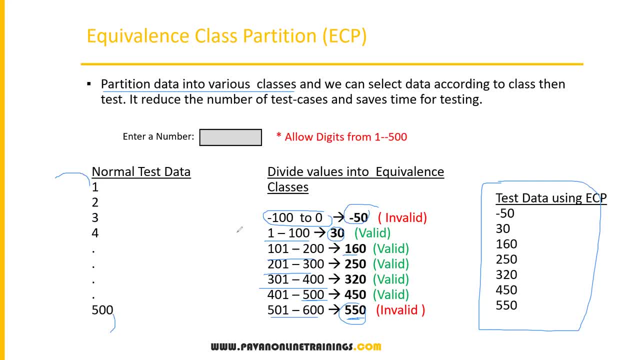 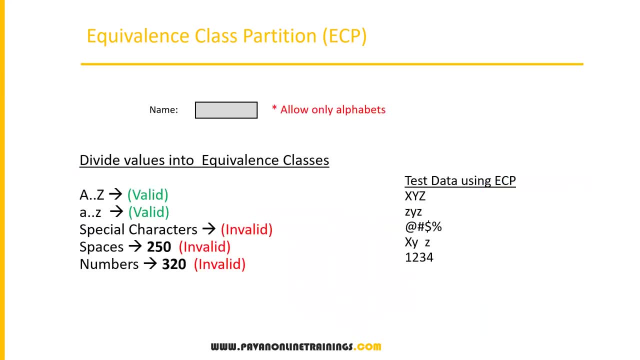 a equivalence class partitioning technique, and now i'll show you one more example. all right, so now look at this. this is also equivalence class partitioning example. so here i have a small text box which will allow only alphabets, which will allow only alphabets, alphabets. 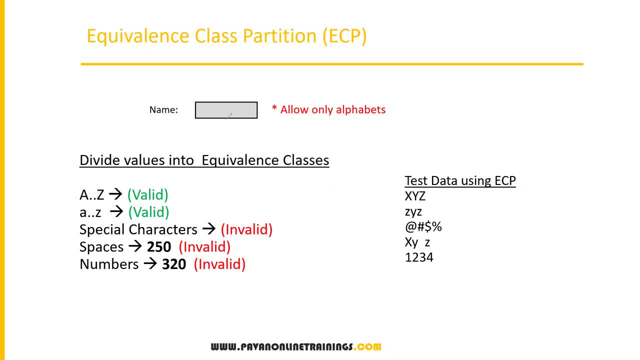 means what a to z, either it can be uppercase characters or lowercase characters. so how we can partitioning the data. so here only alphabets. i'm saying only alphabets means we will partition the data like this: a to z uppercase letters. a to z- small case, special characters, spaces. 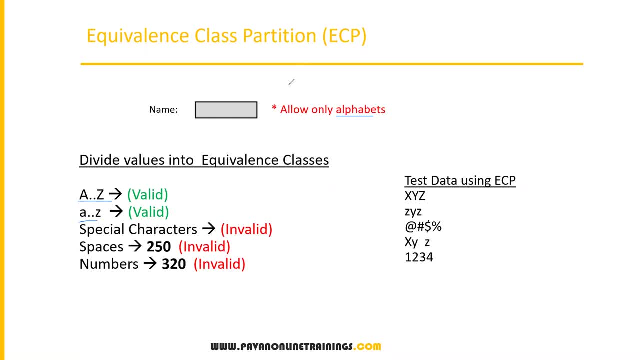 numbers. so this is the actual type of data we have. so now we have to create some test data. so by using a to z uppercase characters, we will prepare some data like this. so from lowercase letters, we use some data like this. and this is uppercase and lowercase is covered now special. 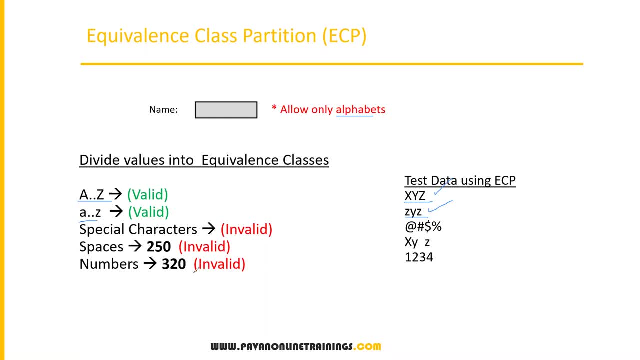 characters are invalid, spaces also invalid, numbers also invalid. so special characters in the sense, these are the special characters. spaces space between the values, numbers. so we first classify the data and then we will prepare some data which is belongs to each and every classification, and this is actual test data which we can use it for testing. 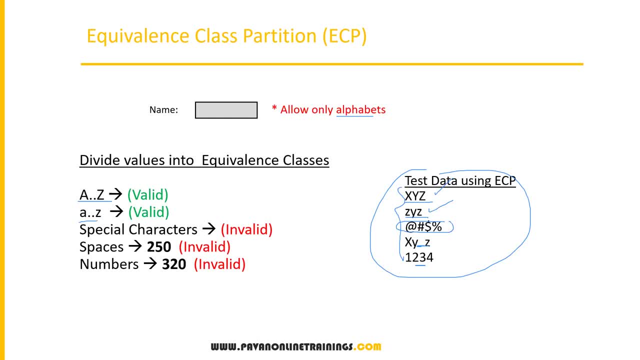 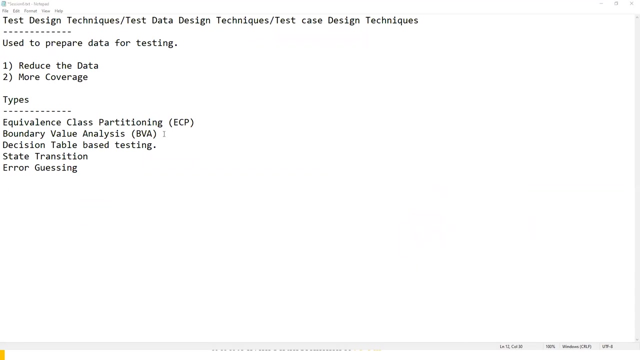 so this is equivalence class partitioning. so in equivalence class partitioning our main intention is the value check what the value we are providing is correct or not. okay, so let me just write a small nodes. so the first technique is equivalence class partitioning. okay, so here shaking the value. or we can say: 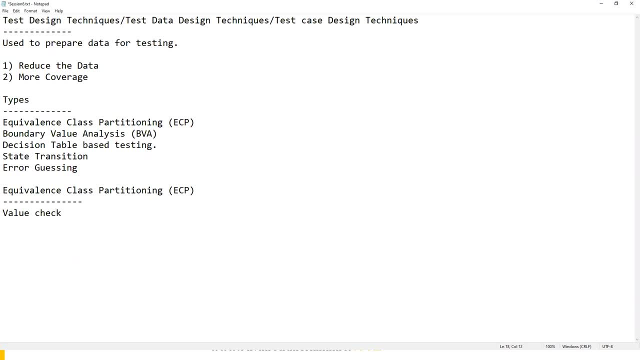 simply, we consider on value check, value check- and we will classify the data data into multiple partitions or multiple classes. classify or divide or partition- any term you can use. okay, so here we are checking the value. you mainly value checking. so we classify or divide or partition the data into multiple classes and 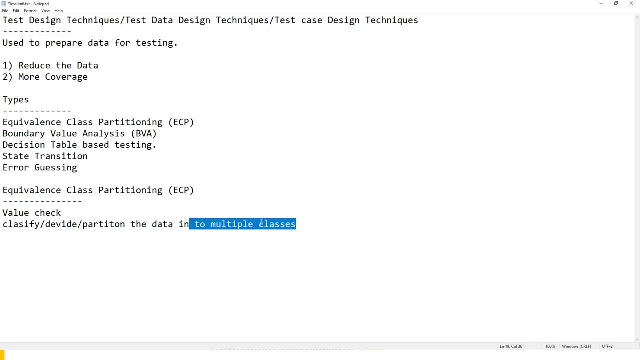 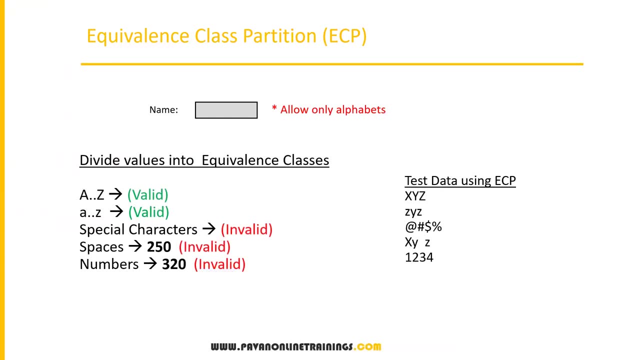 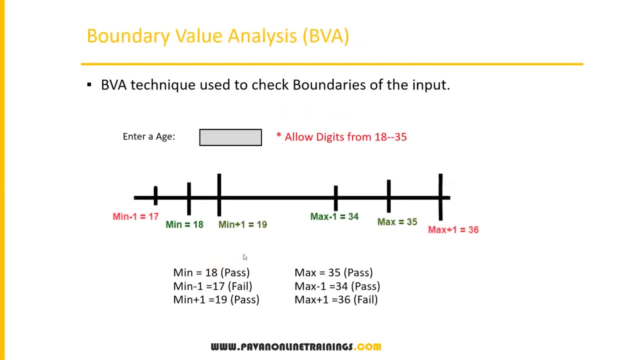 then we will choose data from these classes. so that is equivalence class partitioning technique. this is a one of the very, very important technique which we have to use while preparing the test data. okay, and next one is boundary value analysis. the next technique is boundary value analysis. 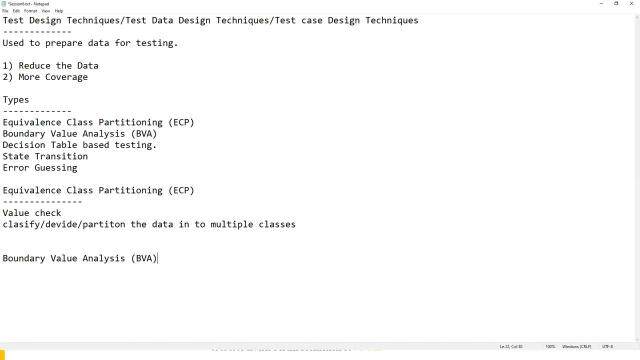 so in the boundary value analysis, we mainly focusing on the boundary of the values, boundary of the values in equivalence, class partitioning, we mainly concentrate on the value. what is the value we are entering in the text field? and in the boundary value analysis we will concentrate on the boundaries, on the value, mainly boundaries we will test, so i'll give you. 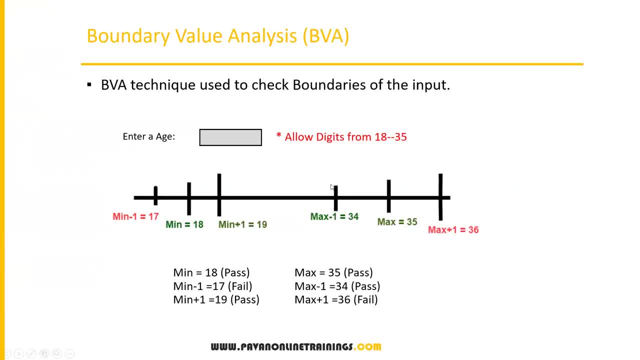 one example. so what is boundary value analysis? so we can call it's a bva technique. so bva technique used to check the boundaries of the input. so, for example, see this: here i have a small text field called age. so here i want to. it will allow us to provide like 18 to 35, so the 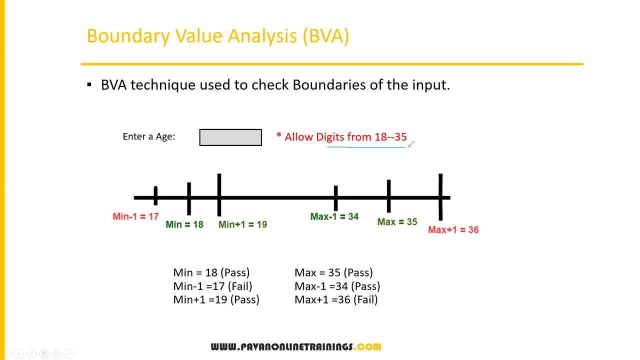 age between 18 to 35. this is my requirement, so normally how we will test it in 18 to 35 means what? when i pass any value between 18 to 35, it should allow. that is all valid data and also i should test it in 18 to 35. it should allow. that is all valid data and also i should test it in. 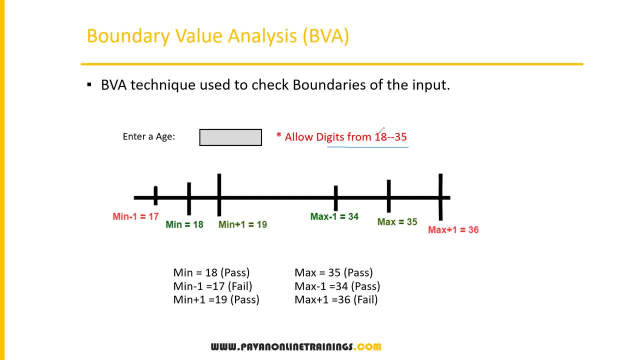 test with invalid data. for that, what i have to do, i have to enter all the values below 18 and also i have to enter all the values above 35, so they should not allow so to cover the positive as well as negative input. so that is a normal way of testing, but in the boundary. 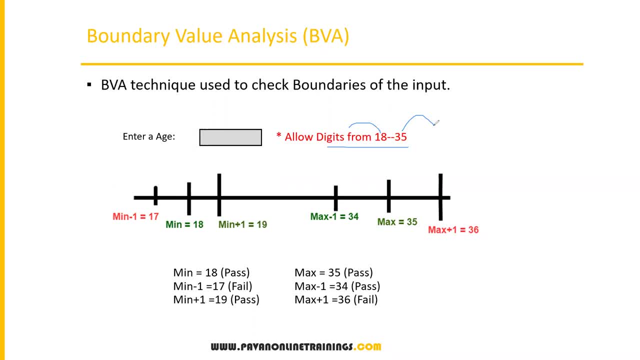 value analysis. we can reduce the data. at the same time we can improve the coverage. but how we can use this technique? boundary value analysis. so in the boundary value analysis techniques, we will just test the only boundaries. we don't test all the values, only boundaries we will test. 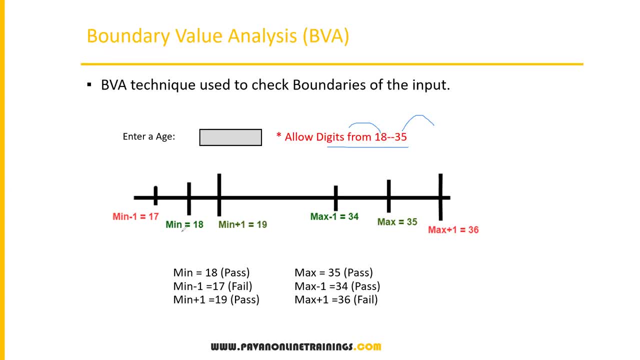 for example. so when i say 18 is a minimum value and 35 is a maximum value, okay. so when i pass minimum value, it should allow. when i pass maximum value also it should allow. and i will test only six parameters here. i will test with only six values, i don't want to test all the values. 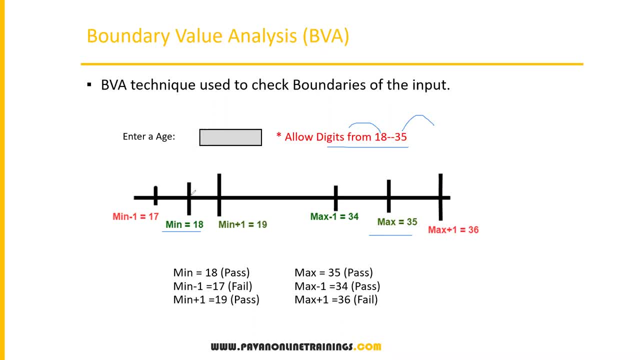 for example, when i pass minimum value 18, you see, it will tell you that if the number of values is, it should allow. when i say minimum plus 1, that is 19, so it should also allow. and when i say minimum minus 1, which is 17, it should not allow. so what does it mean? only three parameters? i'm checking. 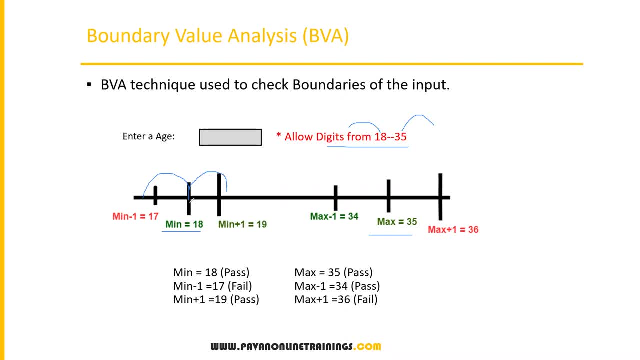 here at the minimum boundary. so when i say, when i pass minimum plus 1, 19, if it is working fine, means what? whatever numbers fall under this particular range should work. but we are not testing all the numbers, we are just testing only one value here. if it is working fine means what? 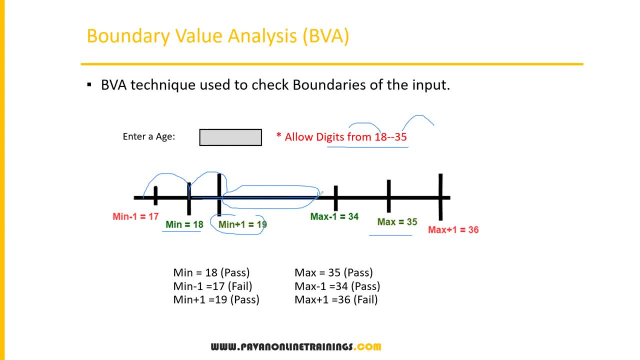 all the numbers between this range will work. similarly, when i say m minimum minus 1, which is 17 and which is not working, means what, whatever numbers are, comes below this 18 will not work, will not allow, because we have just tested only one value below the 18. if it is not working means. 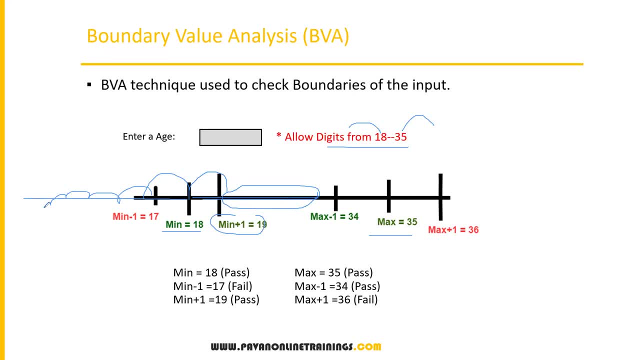 what all the numbers which comes between below the 18 will not allow you. that is covered. and now this is minimum range, minimum boundaries. now comes to the maximum, so max equal to 35 which will allow, and below the maximum number. just, we will verify only one value. 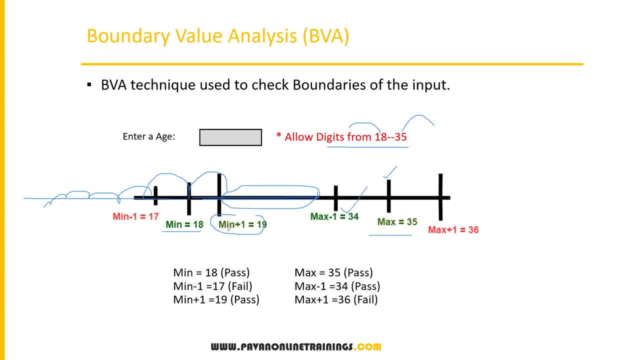 that is maximum minus 1, which will also allow. so here we are checking minimum plus 1, maximum minus 1. so if these, well, two values are allowed, means what all the values will be allowed between this range, now maximum plus 1, and this is suppose between this range and this is minimum: minimum minus one. sorry, maximum minus one. 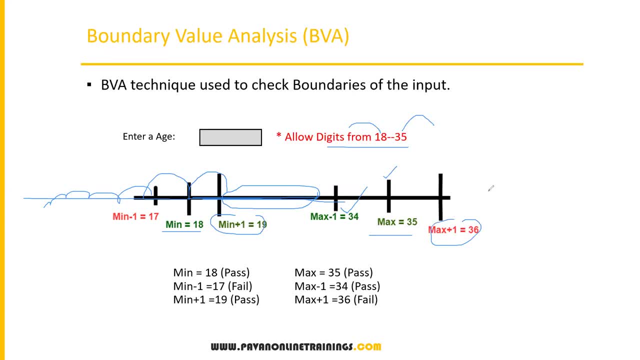 minimum equal to those ones will get, like the minimum 19, into minimum plus one, because maximum minus 1 not valid, not valid so which will not work. if this is not valid and it is not allowed, that means what, whatever number comes after 35 will not allow. so we no need. 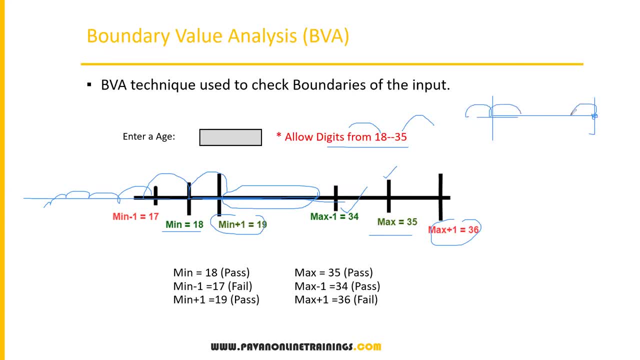 to verify all the values. this is the- comes under boundary value analysis. so in the boundary value analysis we will check the boundaries: minimum minimum minus 1 minimum plus 1 maximum. so this will also reduce the data and the same time it will improve the test coverage. so this is. 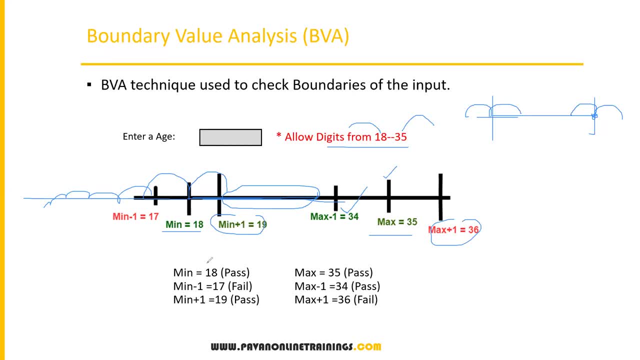 boundary value analysis. so here we will test only six parameters: minimum, minimum minus one. minimum plus one. maximum maximum minus one, maximum plus one. that's it so along six parameters. only two cases will fail. so minimum minus one means this one will fail, and maximum plus one, this get criteria will fail and rest of them should pass. so by taking, by considering this, 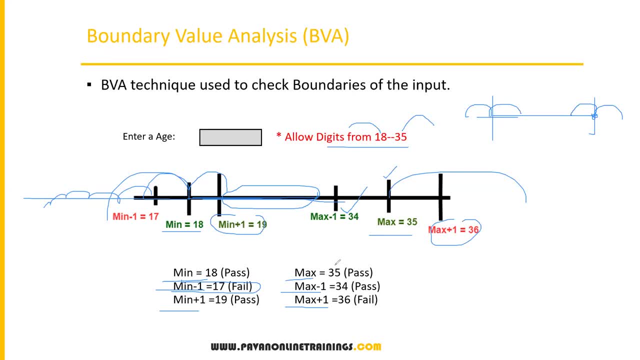 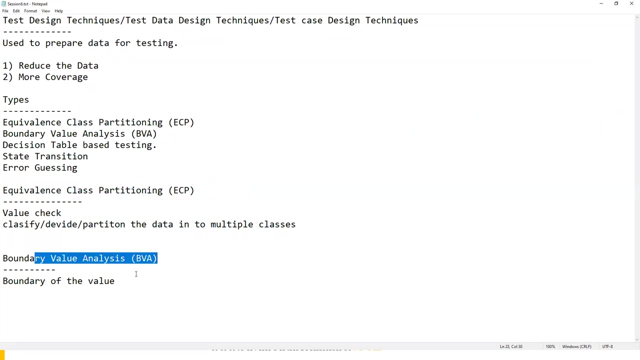 kind of techniques. we can prepare the test data. so boundary value analysis, mainly focusing on the boundaries of the value, not exact value boundaries. i'm talking about boundaries, not the value. okay, so that is boundary value analysis technique. okay, so boundary value analysis, we just verify the boundary of the values and we will consider six, six parameters. one is minimum. 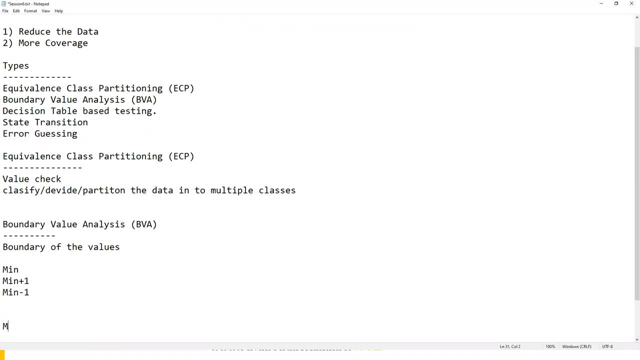 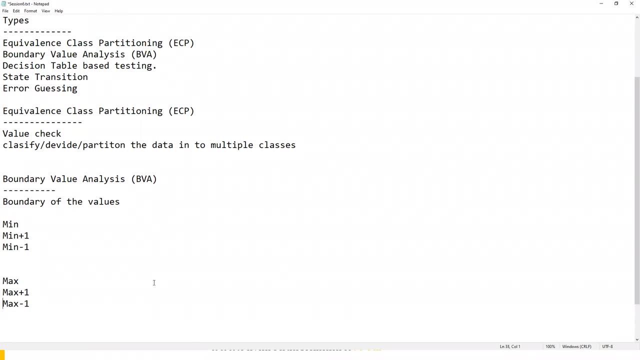 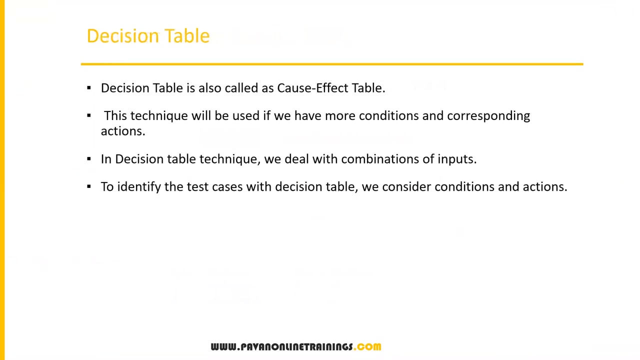 minimum plus one, minimum minus one. similarly at the maximum boundary. so maximum maximum plus one, maximum minus one. okay, so these are the six parameters. we will verify. that's it, that is boundary value analysis technique. now let us move on to the another technique called dation table. so, and one more thing, especially, uh, equivalence, class partitioning. 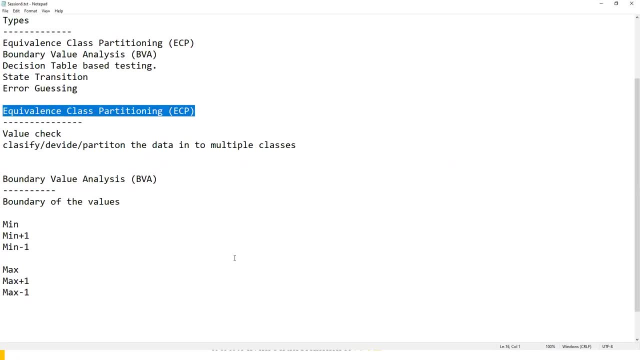 and boundary value analysis. these two techniques will be used in input domain testing. so we have some testing type called input domain testing. so what is input domain testing? means what input domain testing? we will verify the, the input, whatever we provided in the textbox, is correct or not. so the value. 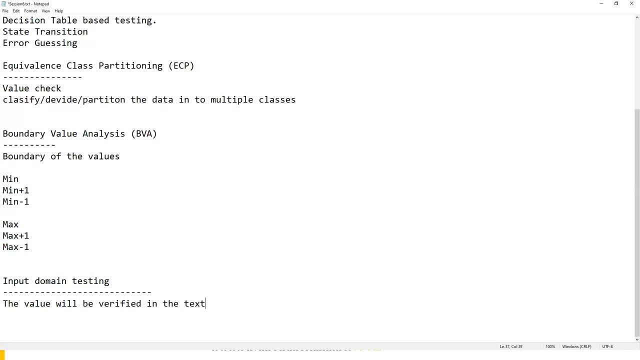 will be verified in the text box, especially text boxes or input fields. okay, then we will conduct the input domain testing, so the value will be verified. whatever value we are providing into the text box, that value will be verified. so, whenever you see the text box where we will apply bva and ecp- ecp techniques to prepare the test data, so the value will be. 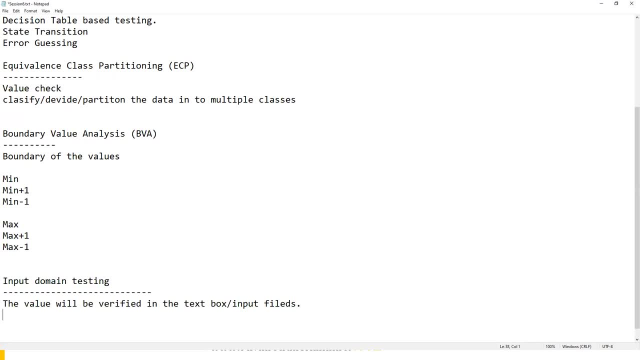 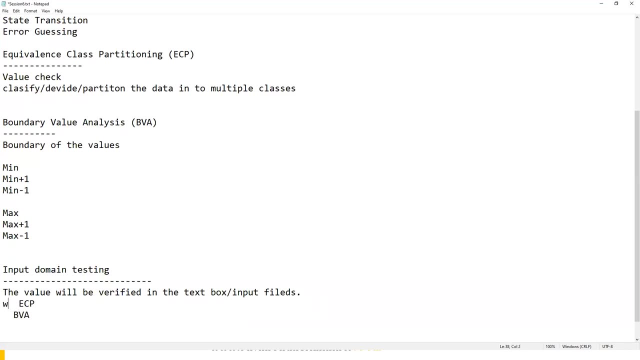 verified in text box or input fields. so here we use ecp and bva technique. okay, so here we use. so we use ecp and bva techniques. so in interview people may ask: what are the input domain testing techniques? so input domain testing techniques we use equivalence, class partitioning and 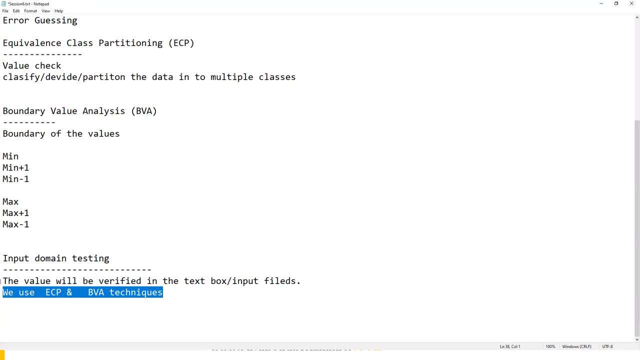 boundary value analysis, which is called as input domain testing. input domain testing means wherever we have to pass some input, where and all we will perform input domain testing. so where we will use ecp and bva techniques to prepare the test data. okay, so the next type. 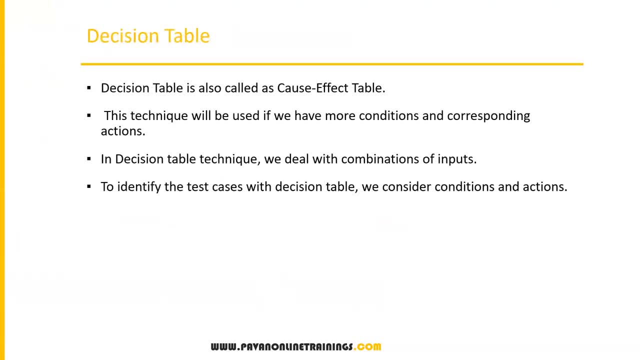 of testing is decision table test, so it is not testing type. actually, don't confuse it. these are not testing types. okay, these are the techniques we use for preparing the test data. okay, decision table. so this is also one of the very, very useful technique and by using these techniques, we can reduce the data. at the same time, we can increase the coverage. 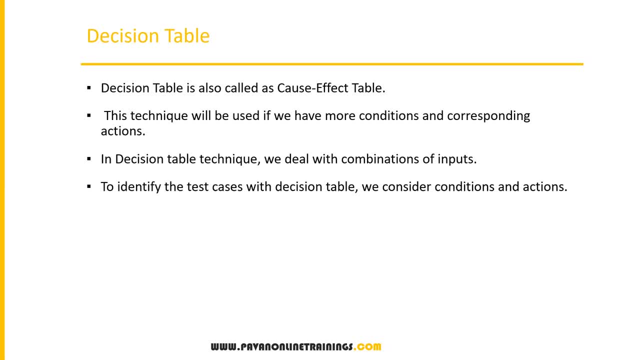 so now, when we use a decision table, and this is also called as cause effect table, cause and effect, cause and effect decision table is also called as cause and effect table, and this technique will be done also when we use not test table in any of these cases. so now, once we know these, 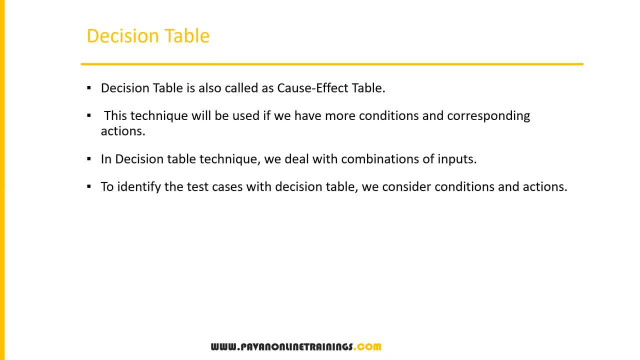 details and we focus towards the scene. so we need to choose Result. how does it work? uh, unless somehow one of our hands is able to traveled. a lot of attention to the camera while working, so on and so on. all right, so you have to socks, subtract one. 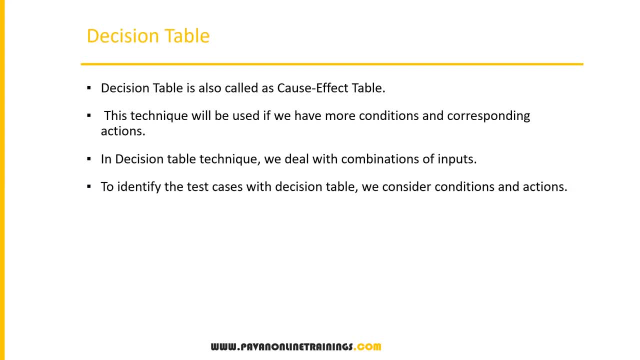 and do the math. now, what you can tell me is: what should we do? uh, at the moment I have a condition and action, so I can just guess the time as such. so, at these times, wait and 음. and also, or do you want to know morebasis preview. 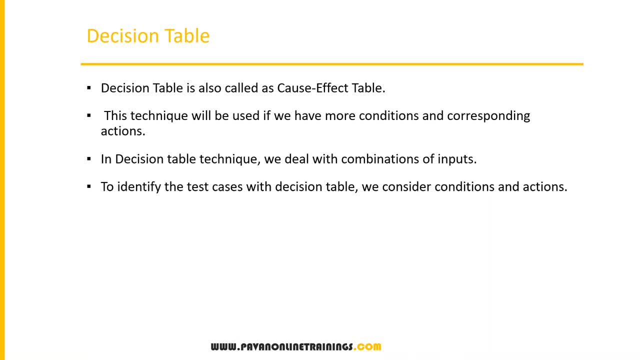 in terms of conditions and corresponding actions. see, sometimes you have certain scenarios where you need time, you have to cover all the actions and for that we have to prepare data. so in that case we prefer decision table technique. so in the decision table, how we will prepare the data. 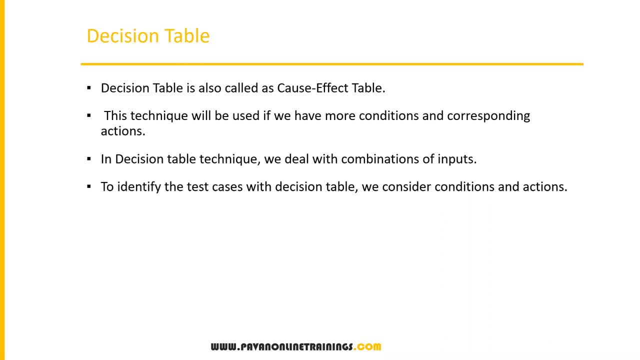 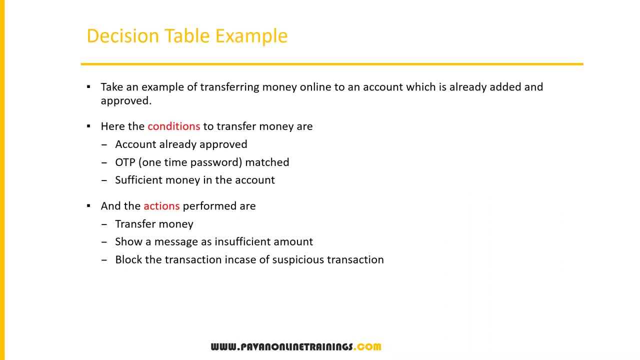 how we can use this technique. so let me show you one example. so this is my requirement. so let's take an example of transferring money online to an account which is already added and approved. so they have one account which is already added and approved account. so i want to send money to that account, and here there are certain conditions and actions. 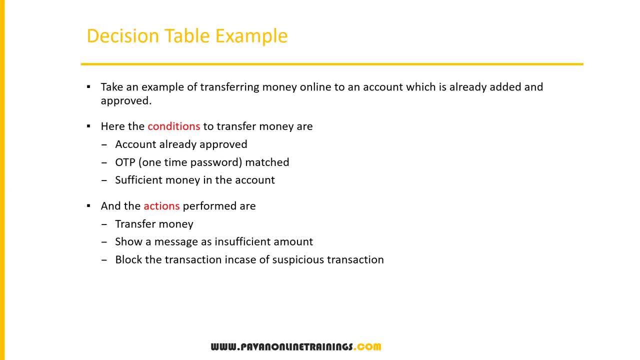 to be performed. so what are the conditions i have to follow? here is so my conditions are okay, so my conditions are: account already approved. account approved- this is one condition. odp matched. so as soon as whenever you sending some money, you will get some opt right that otp should match. 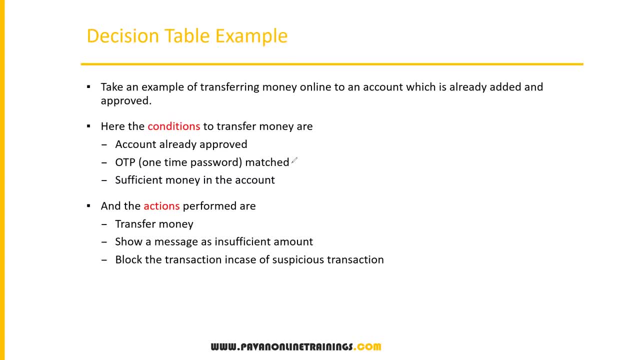 that is one condition. and then you should have sufficient money in your account, okay. so these are the three things you should have if you want to send a money. okay, you are a sender. you have to send the money to the other people, right, they are receivers. so what is the condition, sir? firstly, your account should be appalled approved and otp should be. 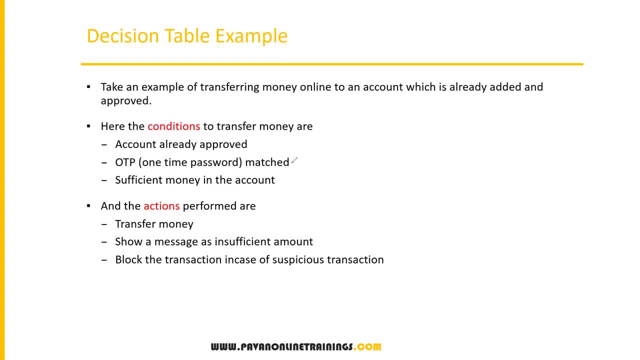 matched and you should have sufficient money in your account. so these are the conditions. should be satisfied now, actions to be performed based on these conditions. we have to do certain actions, so we have to transfer money. that is an action, suppose, if you don't have money in your account, then 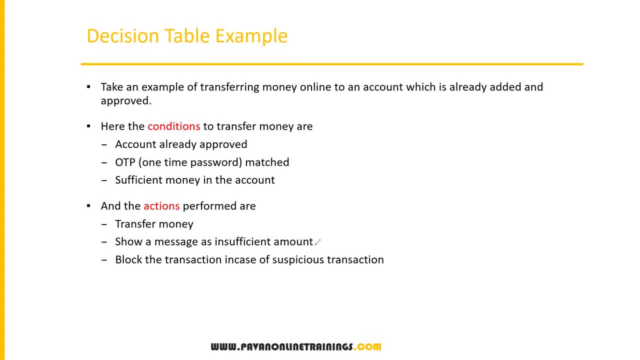 immediately. it should show the message as insufficient amount and suppose: if your otp is not valid or not matched, then block the transaction in case of suspicious transaction. right. these are the actions to be performed based on certain conditions. now for this requirement, we have to write test cases and we have to cover each and every condition at the same time. every. 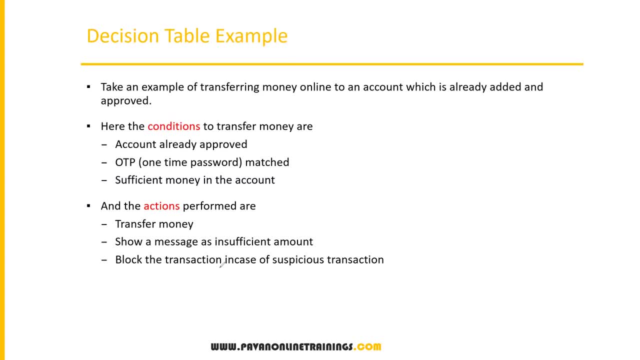 action also should be covered. so whenever you see this kind of requirement, like conditions, corresponding actions, then we go for decision table technique. so now i'll show you how we can use this decision table technique to prepare the scenarios. yeah, all right, so see you in the next session. 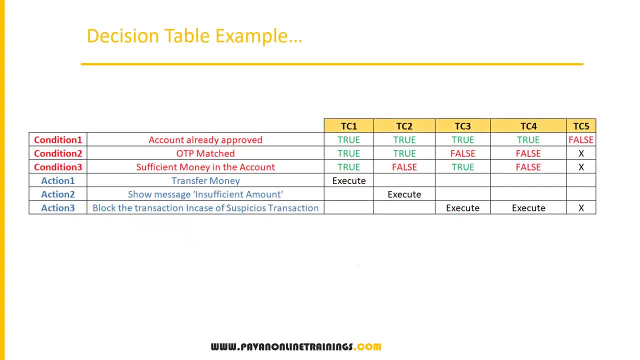 this particular table. so in the decision table technique what you will do is whatever conditions we have and actions we have we will list out in the table. so here you can see. first i provided all the conditions, three conditions. i have again corresponding three actions you have. sometimes you may have a number of conditions or a number. 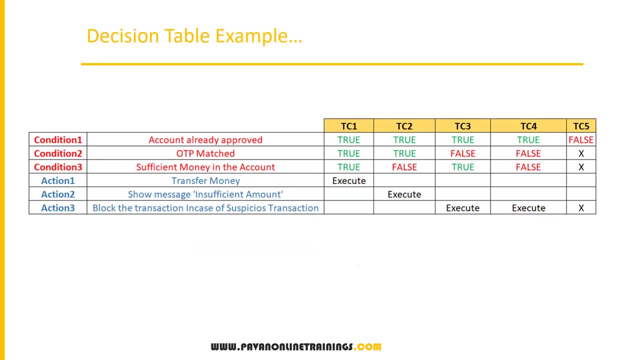 of actions. they may not be equal. so sometimes you have it only two conditions and you have five and five different actions. so first of all, in the particular table- small table- we will put all the conditions and followed by all the actions. now here, if i just look at one, two, three, all three. 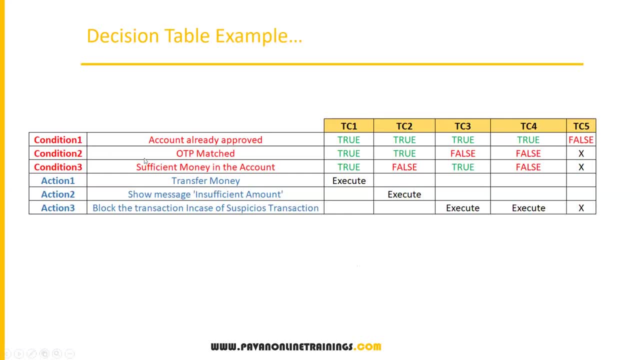 conditions i have put here: account already approved. otp matched sufficient money in the account. so these are the conditions and followed by different actions. so what is action one is transfer money. action two is show message insufficient balance. action three is block the transactions in case of suspicious transaction. so these are the conditions, followed by different. 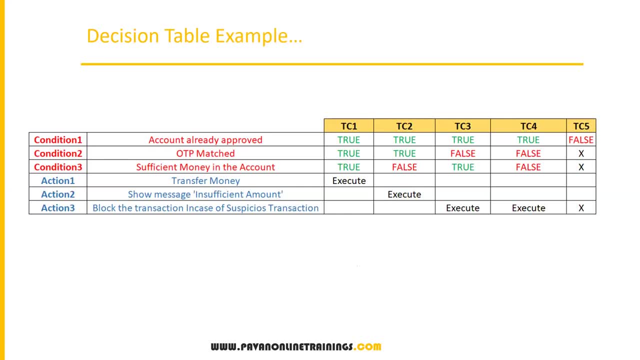 actions. we will list out everything in the table in proper order. so once you provided conditions and actions, then we have to create multiple columns like this, and each column will be one test case, because we need to cover multiple combinations, okay, so here we will mean mainly focus on the 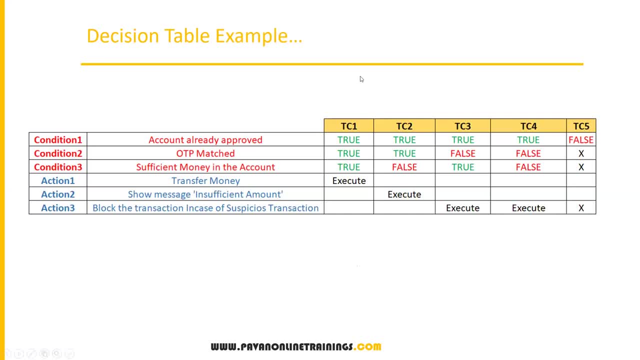 combinations, different combinations of tests. we have to prepare, and we will prepare, multiple columns. we use most of the time excel sheet to prepare this kind of tables. we will prepare, we will add multiple columns like this: each column is representing test case. so this is one test case, second, third, fourth, and you can add any number of columns. 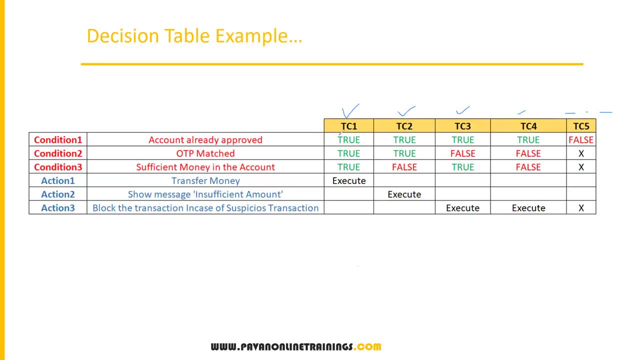 depend upon the coverage. okay, so once you add it, let us check multiple conditions and combinations. suppose account is already approved, which is true, otp is also matched. okay, it is also true. and you also have sufficient account, which is also true. so all three conditions are matched. means what you can transfer the money, so this action to be performed. so this will be. 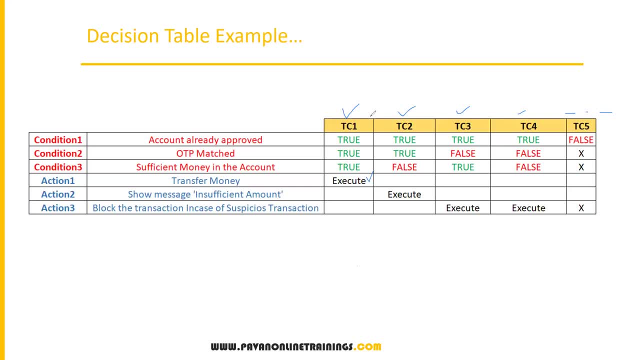 one test case. so your account will be approved. otp match sufficient, balance is enough and you transfer the money. that should be successful. so that is one test case and combination. and the second test case: in the second test case, account is already approved. true, otp is also matched, but 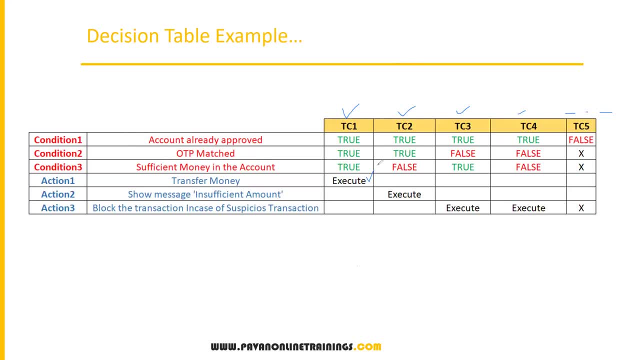 insufficient money in your account. so sufficient money in your account is false. you don't have sufficient amount. then what is an action to be performed? you cannot transfer the money here, right, because you have insufficient money. so show message: insufficient amount. you can transfer the money, but what is the outcome? you 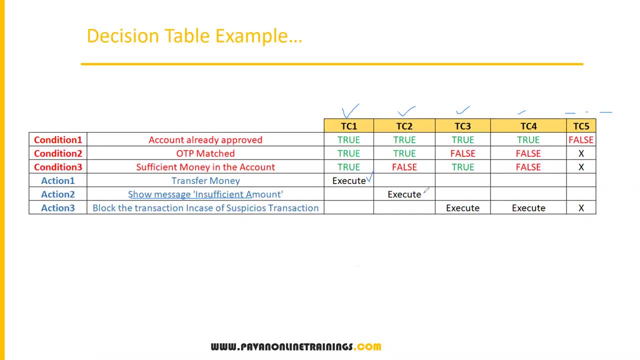 will get. it will cut. so show message in for insufficient amount should be executed. so this is one test case. so account already approved. otp is also match check. you don't have any balance in your account, then try to send money. in that case you will get this measure. show message insufficient. 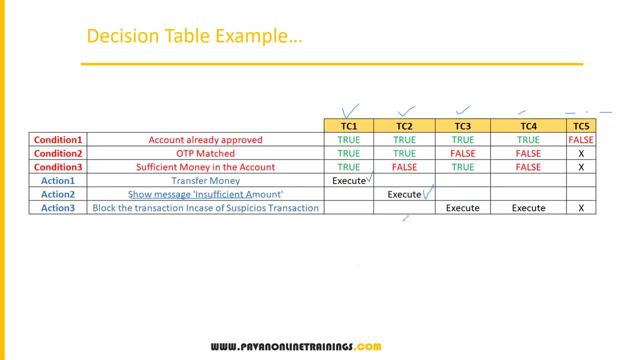 account, you should be executed. this is the one combination. now the next combination: account is already approved, otp is not matched. you also have sufficient money in the account, but otp is not matched. and at the time when you send the money, what will happen? block the transaction because 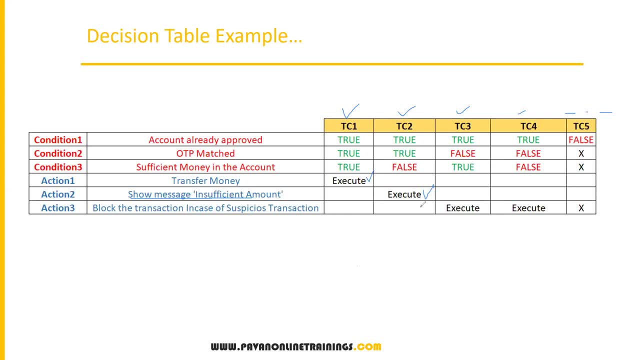 otp is not matched, so block the transaction in case of suspicious transaction. this is one test case, so you need to mainly focus on different combinations, act condition and corresponding actions. now the fourth test case. so account is already approved, which is true, but otp is also not matched. there is no sufficient money. otp not matched, there is no sufficient money, then what? 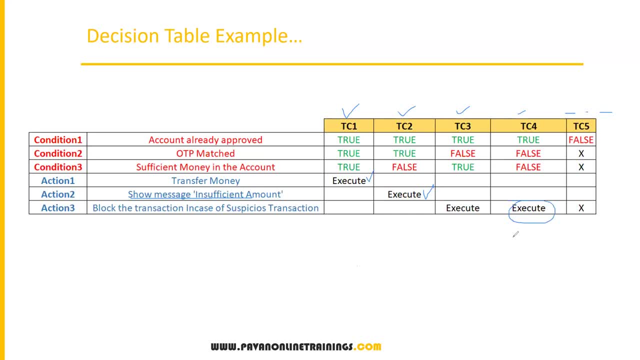 happens again, the last action should be executed. block the time because otp is also not matched means block the transaction. this is one test case and only the first one is a valid test case. rest of three test cases are the invalid or negative test cases. we know we don't say invalid test case, they are negative test cases. 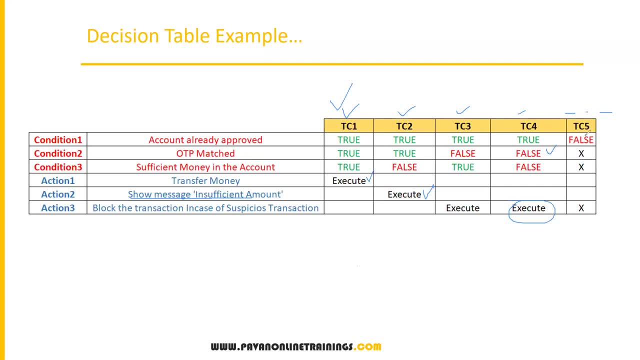 and the last test case is actually invalid test case. suppose account is not approved. when i say false means account is not approved. account itself is not approved means there is no chance of otp matched or having the sufficient money, right. so this is an invalid test case. this is an. 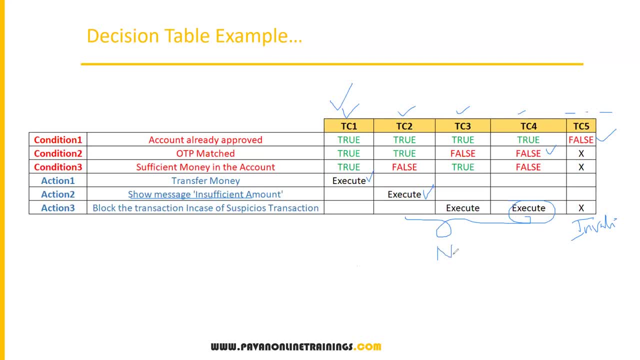 invalid test case. and these three are the negative test cases and the first one is a valid test case. okay, so based on this table, we can prepare the test cases by which we can conduct the testing. so here we covered all the combinations. the account is up, already approved, but otp is not. 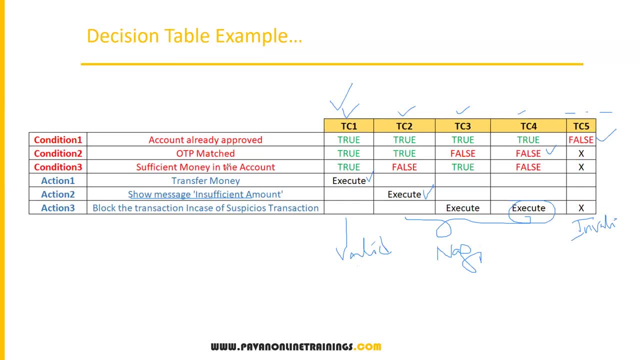 matched, sufficient money in the account is not there, then what is action should be performed? similarly, account is already approved, otp not matched, then what is action should be performed? the account is matched, otp is matched, but insufficient money in the account. and what is the action should be performed? so by using this, 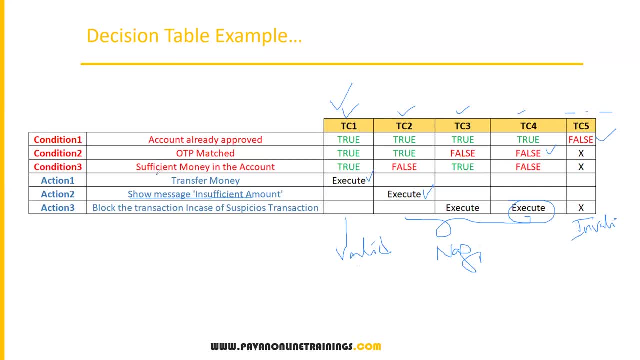 decision table, we can cover each and every combination. okay, so conditions and action should be there. so, whenever you have number of conditions or more number of conditions and corresponding actions, and this technique will be very, very useful to prepare the test data along with the test cases. now every column is one test case, so for, based on this column, we will prepare 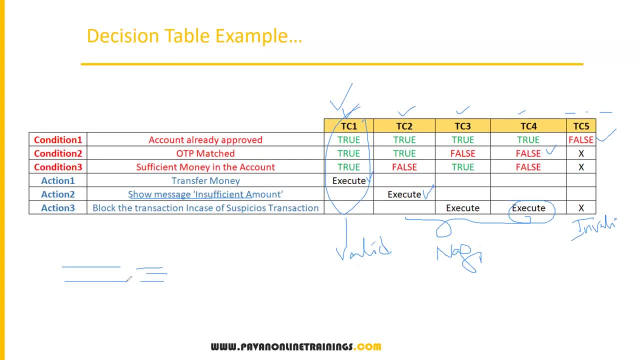 some tests. okay, account is already approved. otp is matched. transfer the money, sufficient amount in the money and transfer the money. these are the steps to be written, execute and then what is expected like money transfer should be successful. so this is actual test case which we have to. 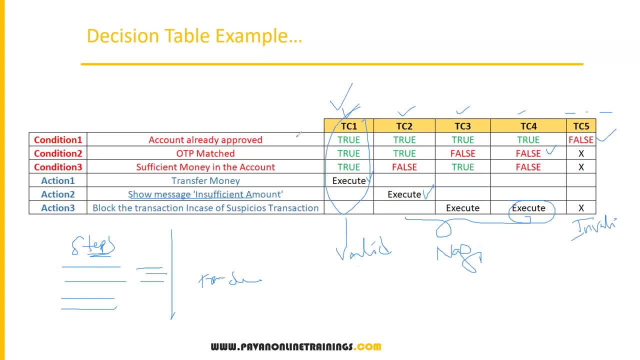 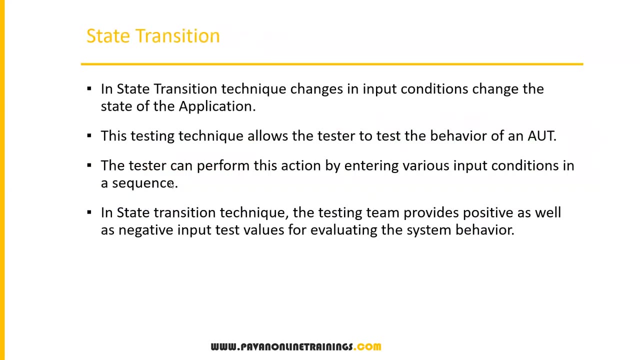 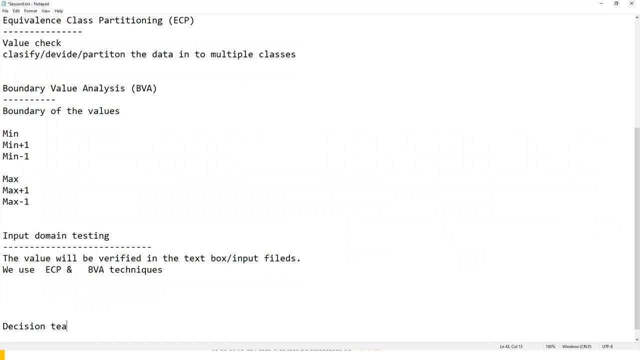 prepare based on the columns. okay, this will cover each and every combination- okay, of the data condition corresponding actions. so this is a example of decision table. now the next technique is state transition. so let me write some nodes decision table: if we have more number of conditions corresponding actions, then we use decision table technique. so in 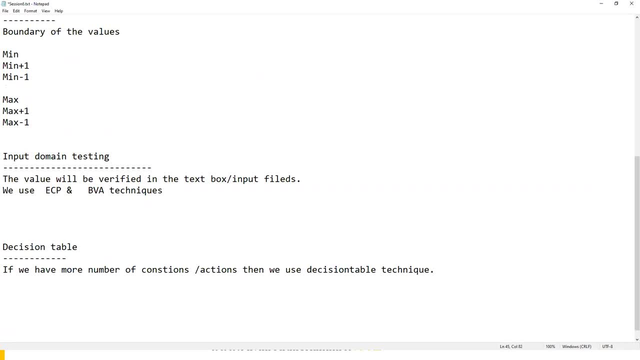 interview. people may ask when you have to use decision table technique. can you give him one example? then you should able to explain with some example. so draw some picture. take one small requirement like this- i have given one example right. so take small requirement and try to design. 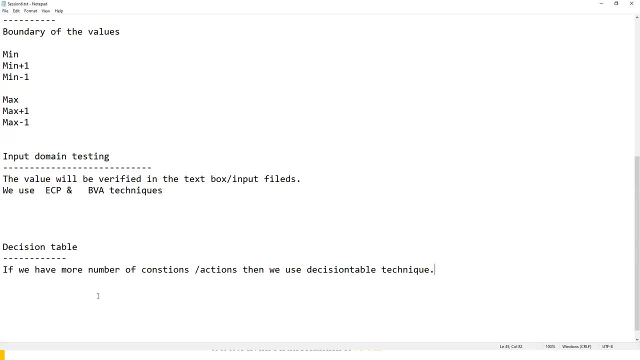 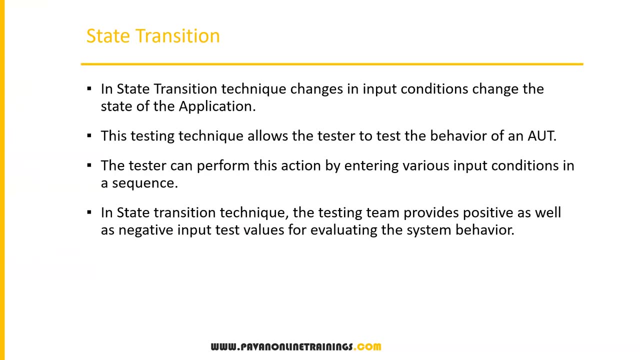 the table and explain in proper way. okay, so this is a decision table. now, state transition is also one of the technique which we use for test data designing technique, so let's see what exactly it is. so state transition is a technique. uh, basically, in this uh input will be changes based. 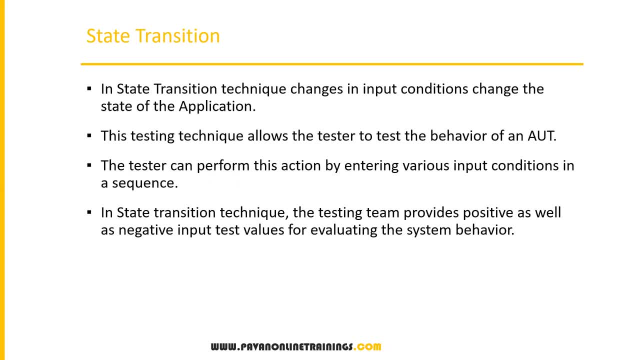 upon the status. so we will do different navigations or different actions and accordingly input conditions also will be changed. i'll tell you one example, then you can understand. so this tactic i'll allows the tester to test the behavior of application, and the tester can perform this. 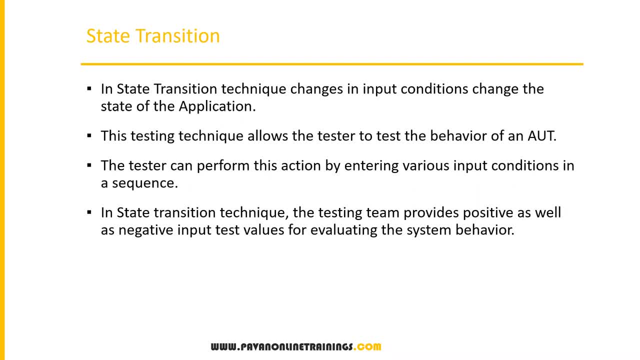 action. by entering values, input conditions in a sequence manner and in state transition technique. the testing team provides positive as well as negative input test values for evaluating the system behavior. so first let us understand what is state transition. state transition means what? changing the state from one to another, changing the condition from one state to another state. 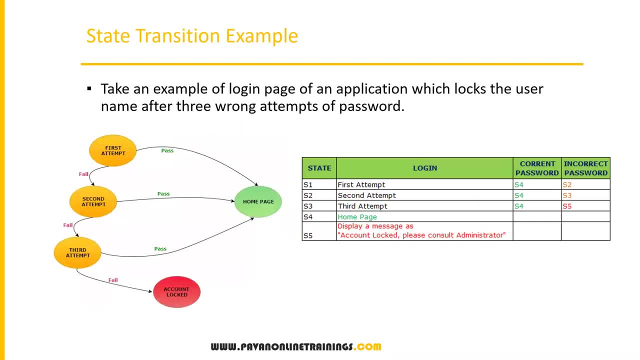 so let's see this example and this is something called a login part. suppose if you go for an atm or if you are using internet banking application. how many times password allowed. suppose if you enter password wrong, how many times it will allow maximum three times right, even if. third time, if, 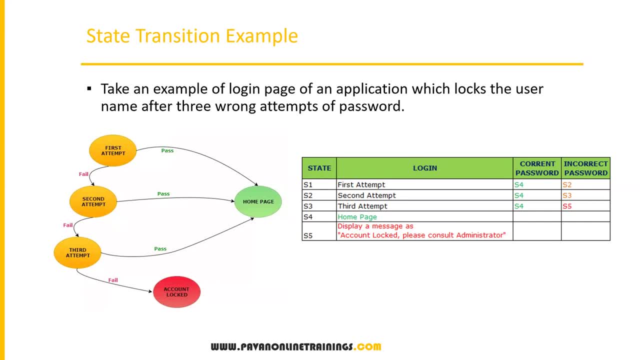 enter password. third time is also: you enter is a wrong password, then it will lock or it will block the account, right? so let us take that scenario and see how state transition example works. if i just look at this, i have a small picture. so take an example of login page. 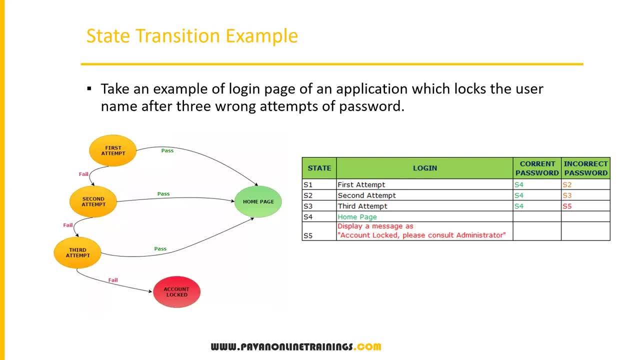 of an application or some atm which locks the username after three wrong attempts of password. okay, this is my requirement or scenario. now let us first we need to check the different states. so let us first check the different states. so let us first check the different states. so when i enter the password first time, when i enter the password first time, it should allow. 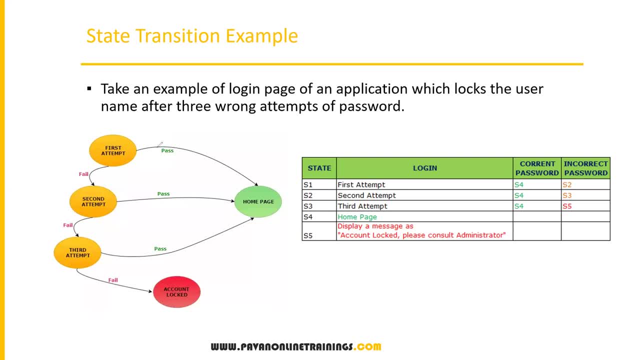 if it is a correct, it should allow. okay, it should pass first time. if a proper password is provided, it should allow and it will give you home page. and here what is the transition? so we are there in the login page and first attempt which is valid password and then home page is displayed. 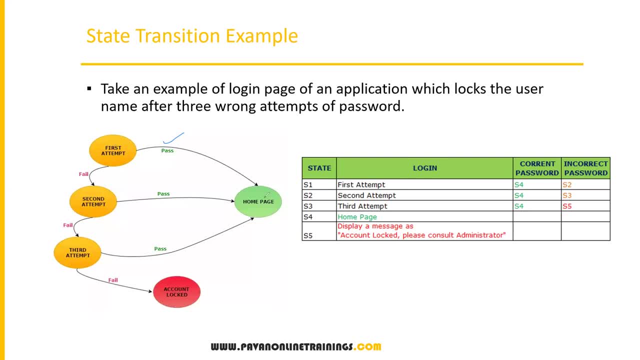 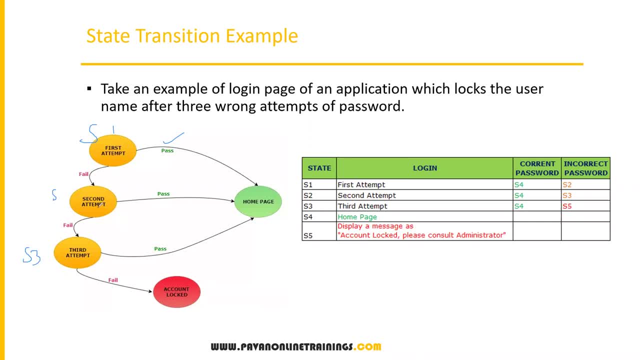 two and this is a state three. so each and every attempts we consider as a states- state one, state two, state three- and in every state we provide some kind of input- valid input and invalid input. so valid and as well as invalid. if i provide a valid input for this state, it will go to home. 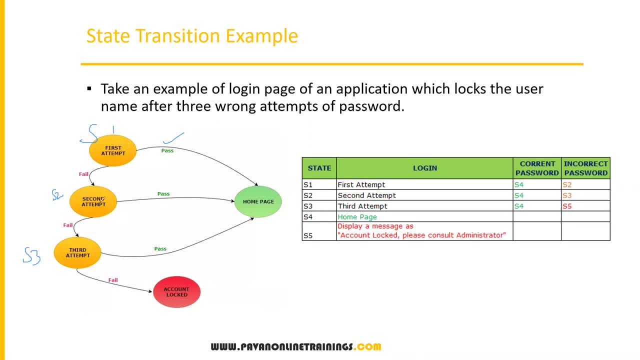 page. when i pass invalid input, it will go to the next state. similarly, if i pass valid input, it will go to home page. we pass invalid input, then it will go to next state. so by changing the states, we are also providing the valid input and invalid input. so, based on this diagram, we will prepare a 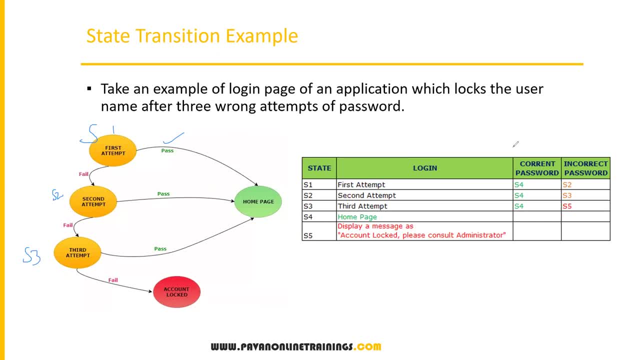 small table like this, and this will give you more clarity on this. so first, we will have all the states, so there are multiple states we have, so even this is also state. let's say we can call it s4 and this is a es5. this is the. every node is representing the different states. now we will list out all the. 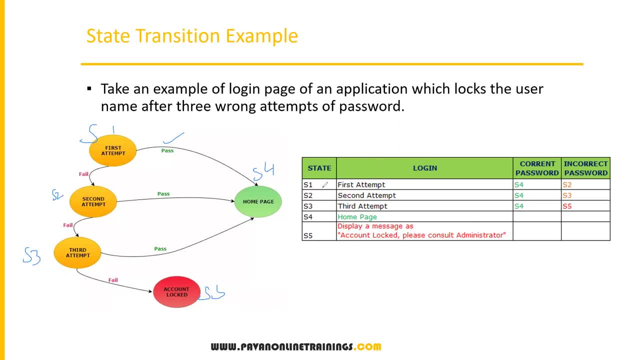 states in one column and we will also name them. s1 is a first attempt. s2 is a second attempt. s3 is a third attempt. s4: display the home page. s5- account is locked. so five different states we have specified, and then here we prepare some data, suppose in the state, one in the first attempt. 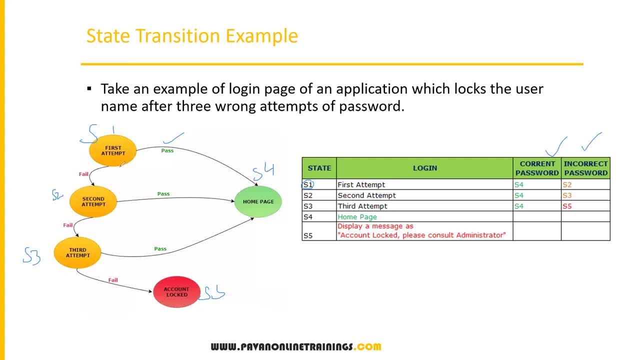 we pass the correct password. when i pass the correct password, for example in this state, I confess the course password and then in which state we have to go. it's four. if I pass the correct password in the state, one we have to go to is 4 s 1, 2 s 4. so if I pass the correct password, then we go to s4. 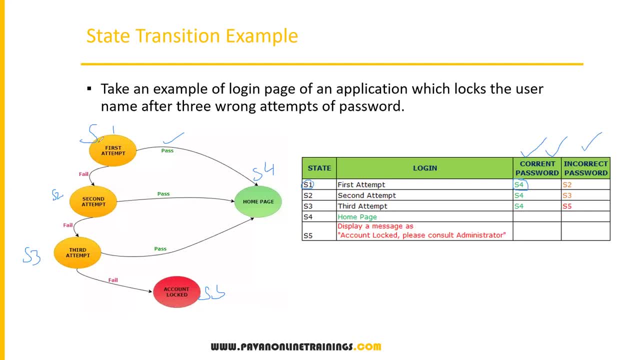 if I pass the incorrect password here, then we go to another state. what is that here? s2, that means second state. so if i just look at the first row here in the first state, if i pass the correct password then we go to s4 state. that is home page. if i pass incorrect password in the first attempt, it will. 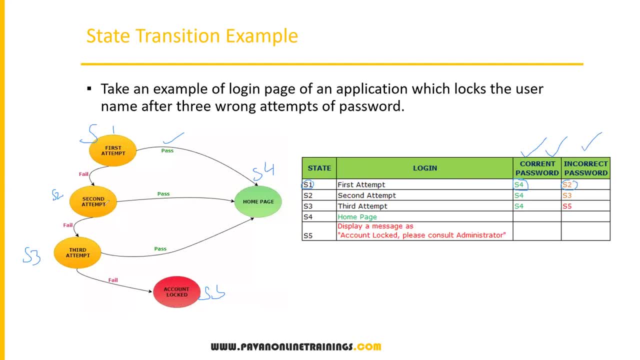 go to s2. s2 means what second attempt. so this is the one test. now the second test, second attempt: s2 representing the second attempt in the second attempt. if we provide the correct password in the second attempt, if i provide the correct password, it will go to s4. so s4 and in the second attempt. 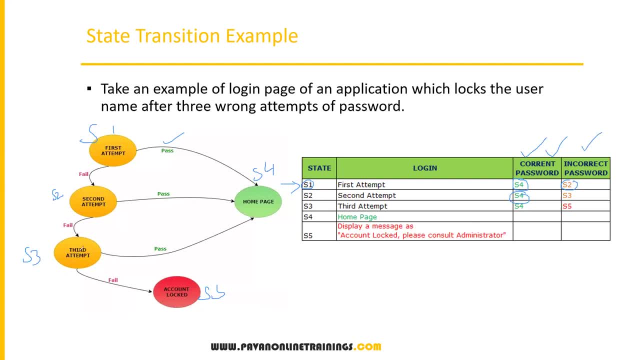 if i pass an invalid password, then it will go to s3. that is a third state. this is a one test. now s3, state three. in the state three third attempt, if i pass the correct password, it will go to s4. so s4, this is valid. 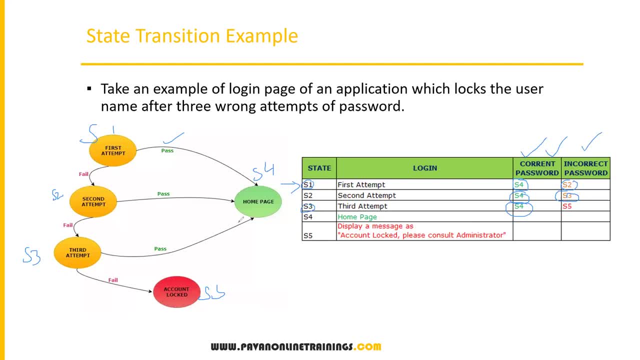 in third attempt, in s3, if you pass invalid password then it will go to s5, that is, account is locked. so this is a straight transition: one state to another transition how it is going to change based upon the input we provided. based upon the input we provided, when a pass valid input and 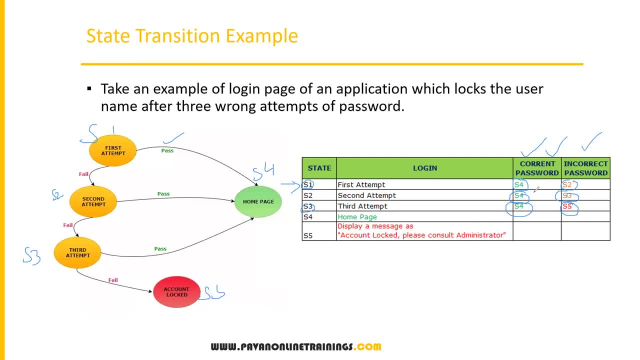 invalid input, how the state is transferring or how the state is transitioning one one step to another step, so that we are going to focus on the second step of the third test. so this is another technique which we have to use: state transition example. okay, so if you have multiple navigations, 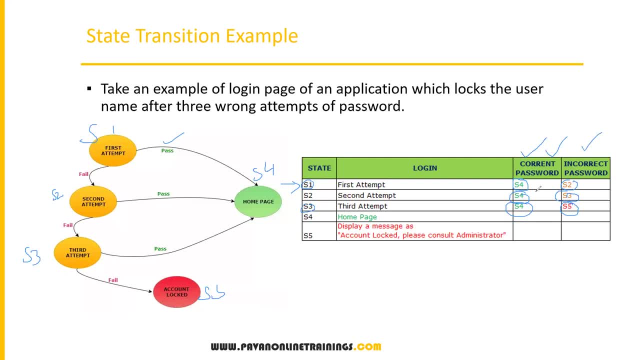 and where we have to pass valid as well as invalid data and then we check whether properly working application 100 test which is properly working or not. so this is a one of the important technique, state transition technique. so decision table will be used if you have more number of conditions and corresponding actions. 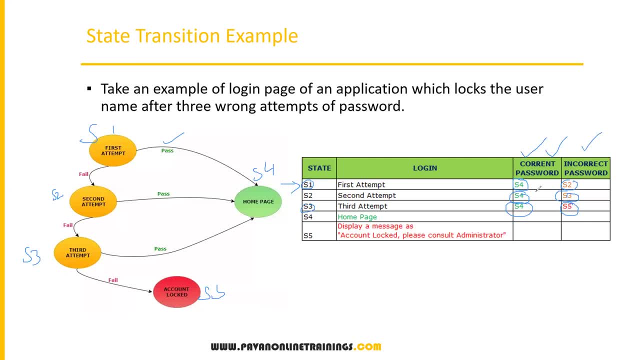 and the stage transition technique will be used if you have a multiple conditions, not conditions, multiple states. here we mainly focus on the different states of transactions, like different atoms, okay, so remember this. and the last technique which we have is error guessing, error guessing. okay, this is a very simple, a small technique, and we don't have any, uh, something, any. 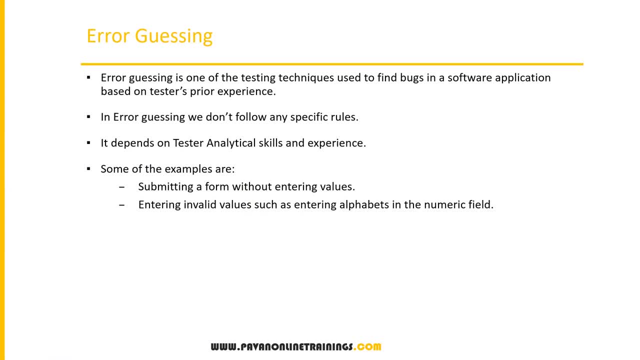 conditions, actions, nothing. it is just guessing the error. so when you will able to guess the error? so, normally, if i give some application, okay, and something is not working, how we will know that whether it is working properly or not? so, based upon your guessing, based upon your experience, 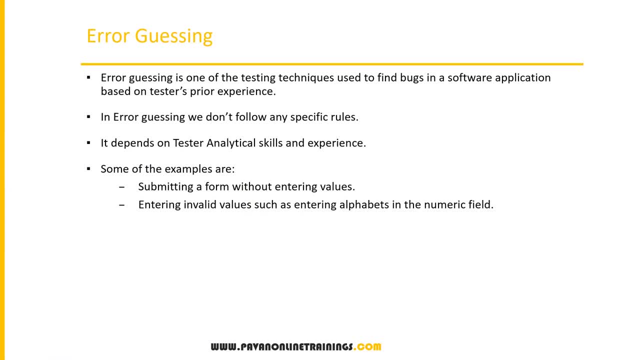 based upon your analytical skills, you will be able to guess the error and you will be able to right, and this is purely depends upon the tester individual analytical skills. based upon their experience, they can guess the error. they can guess the error. for example, you have some online. 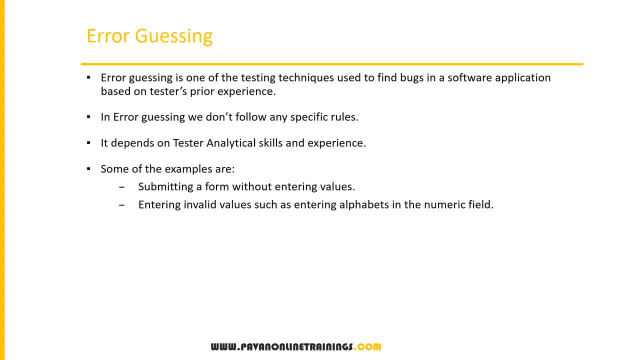 applications. so where you want to set the products, add them to cart and then you do payment. okay, this is a flow. first we need to search the products, add that product to your cart and go to the cart and view. so this is the action flows. so suppose you don't have any test case or any document, nothing. 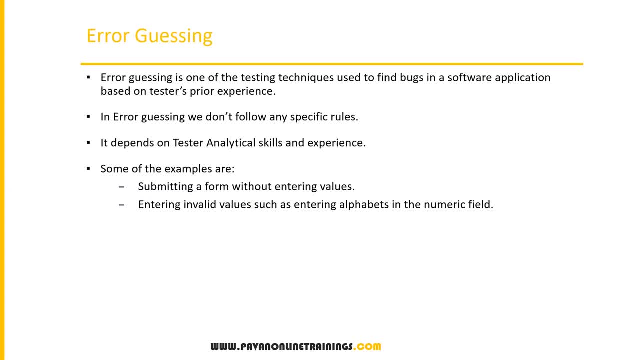 and i'm searching the product and after searching the product and adding to the cart, and then there is some payment options are not properly working or payment is got failed, then immediately you guess it. okay, there is an error in the payment process. or suppose whatever product you selected, 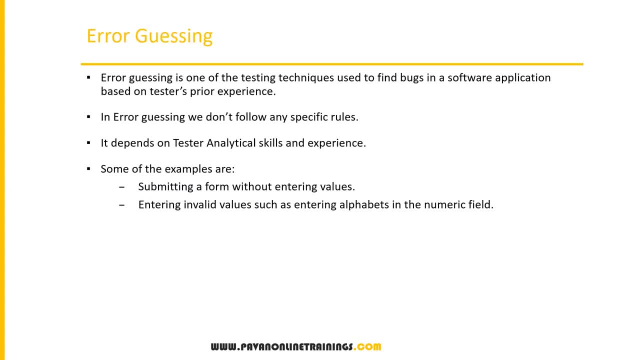 when you click on add card, which is not properly adding to the cart, will know that. okay, this is an error. and do you refer any documentation or do you refer any other document to do to guess this? no, this is just our assumption. this is our, just our- analytical skills. 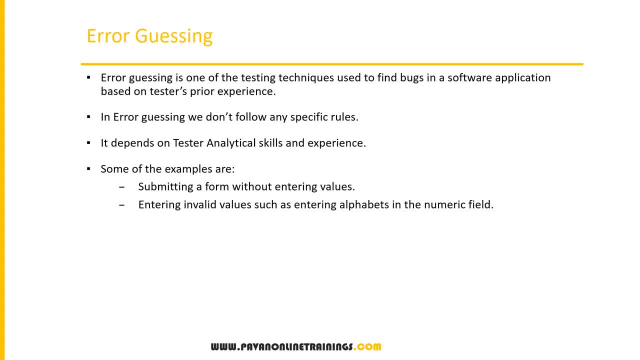 this is just based upon our experience. we can tell where this is error or not. okay, this is purely depends on the tester analytical skills and their experience. okay, so this is error guessing techniques. whenever you do some testing or actions, you can guess. maybe this may be the. 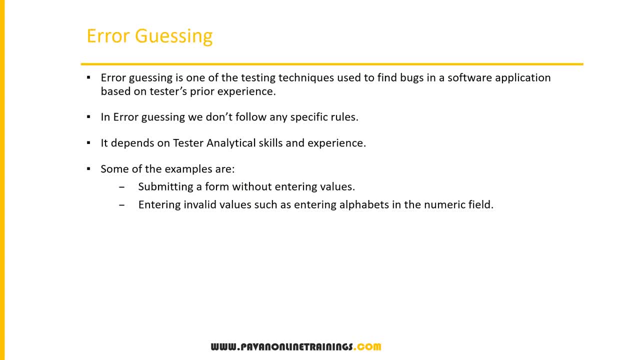 error, or this may be the not error. you should able to judge it okay based upon your analytical skills and your experience. that is basically called as error guessing. so error guessing is a one of the testing technique used to find the bugs in the software based on the tester's prior 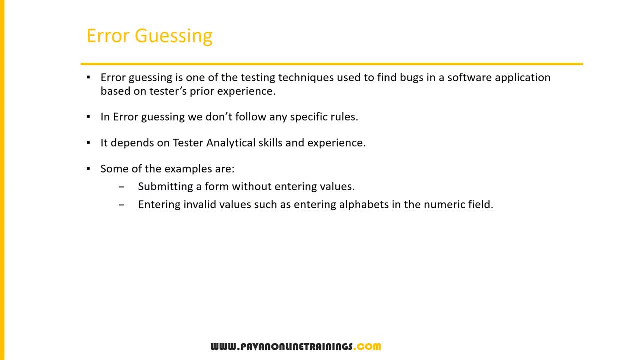 experience. so error guessing. we don't follow any specific rules and regulations, nothing, just we are blindly test the application and check the errors. this is also one of the technique and it depends upon the purely tester analytical skills and their experience. okay, and some principles we follow here. 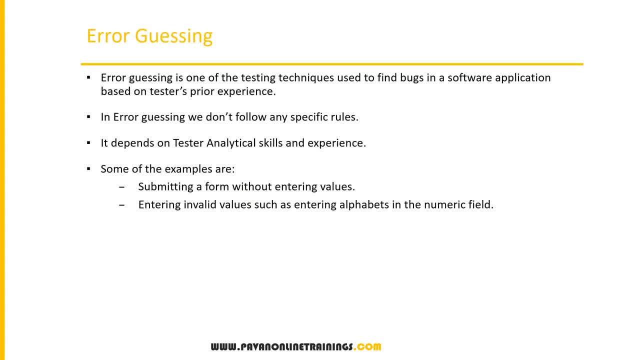 some examples are, let's say, submitting the form without entering a value. so what you will expect? i don't have enter any value in the form, but i'm just click on the submit. so there should be some error message should display, and that is a error. we are guessing. we are expecting some error should. 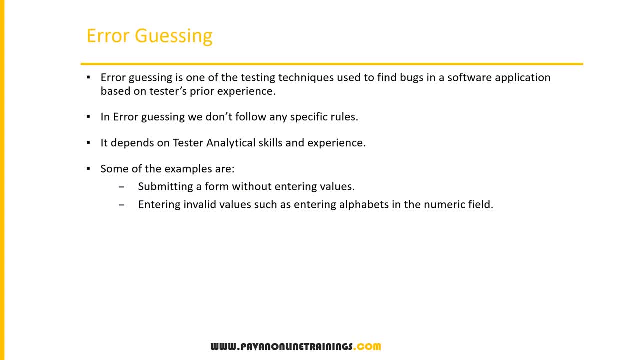 be there. so that is called a error guessing. similarly, entering some invalid values in the text boxes. okay, entering invalid values, such as entering alphabets or numeric fields, combinations, and what kind of error it is getting? suppose you have some box and it allows only numbers, but you enter some text or you enter some alphabets. you are expecting some error, right? and 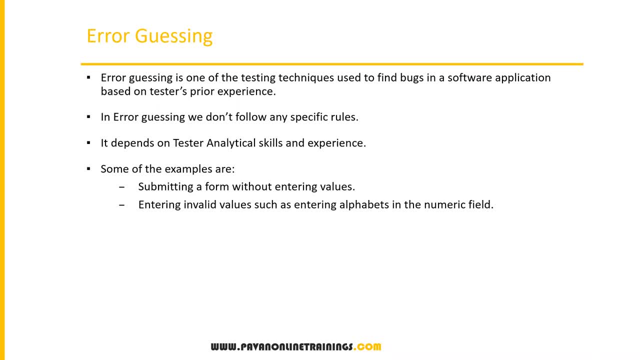 similarly, suppose i have a uh numeric field. they have some number but they have no numeric field. so it will allow only numbers, but you have entered some alphabets or special symbols, something like this. so in this case you are guessing some error, you are expecting some error from the application. 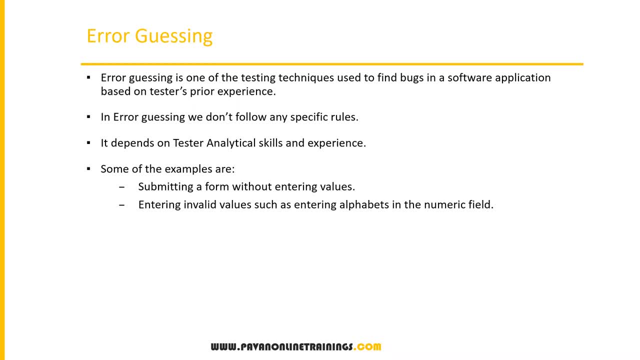 so that is called as error guessing. that is called as error guessing. so in every area we can get some error. we can pass some invalid data and check the error is coming or not. okay, that is a error guessing technique. so these are the six techniques which we have to use. 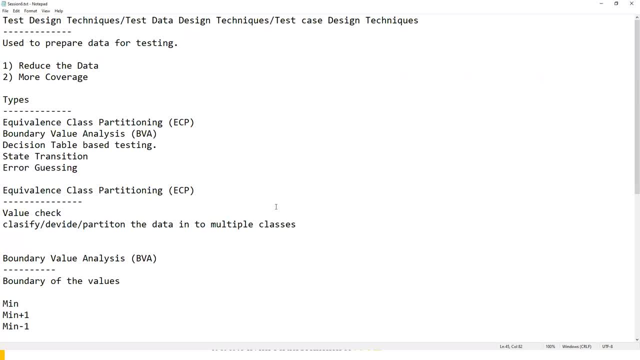 to prepare the test data or test case design. so equivalence, class partitioning, boundary value analysis, decision table testing or decision table is one of the technique and state transition and error guessing. so these are the five test design techniques which we have to prepare test cases or test data, and what is the use of these techniques which will reduce the data? so 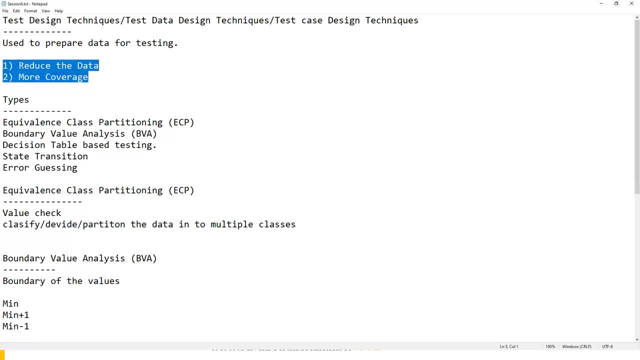 this is the main focus we have to. okay, you need to focus more on this. why we need to go for techniques. if you don't use techniques, you will prepare huge number of data and they may not cover- they may not cover- each and every scenario in testing. okay, so you have to prepare the data intelligently so you have minimal test. 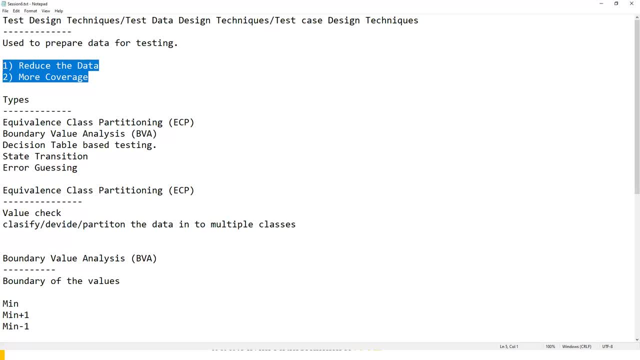 data at the same time. it should cover everything. you should not miss even a small corner scenarios while testing it. for that we need to prepare different combinations of data. so so the main usage of testing techniques is reducing the test data. at the same time, we increase the coverage of testing. so coverage is very, very important in all the 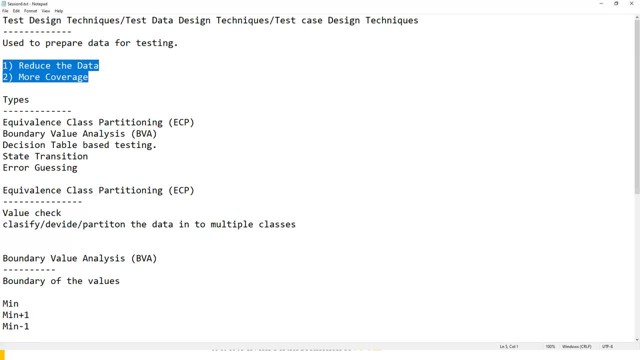 cases as a user, even though i'm a tester, i should always think about the user. so if i give application to the user, what kind of data he may enter? so we have to think in the user perspective and think all the positive and negative test cases, all the positive and negative scenarios.